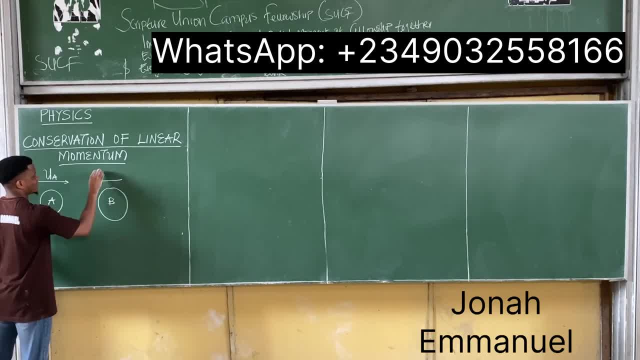 And then body B moves in the opposite direction with, let's say, U, B, that's velocity of B. Now, when they collide, all right, when they collide, you have: this is before collision, this is before collision, okay. When they collide, you have something that looks like this: 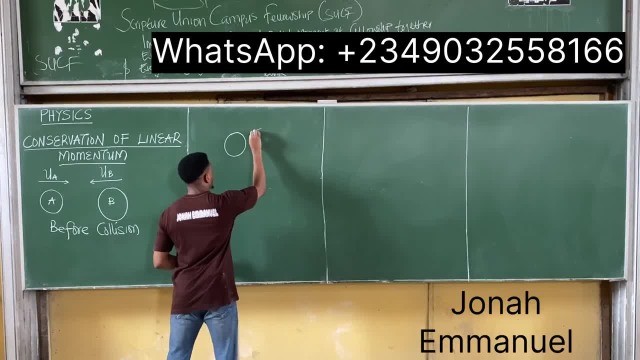 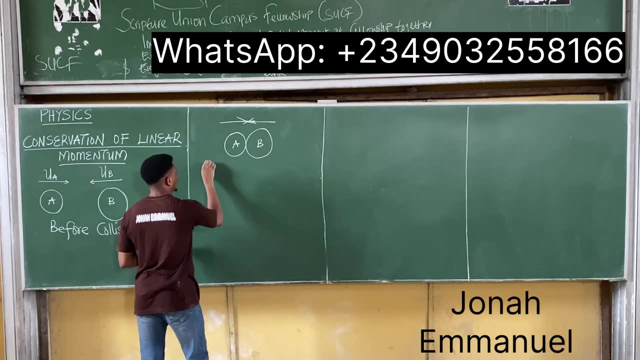 body A and then body B, like this: This is A, this is B. Now have these two hitting up against themselves like this: all right, So this is, this is collision, like I said during collision. okay, So during collision and hit against. 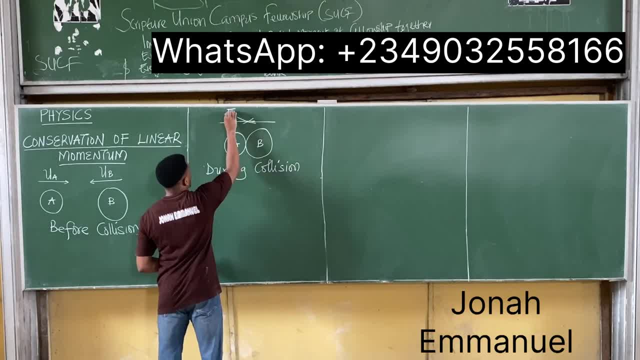 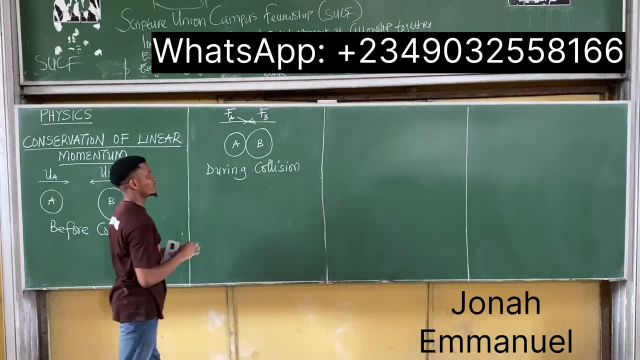 themselves. Of course, this is hit this with a force. let's call the force F A. B also hits A with its own force. let's call this F B. all right, So they collide. this is during collision, When they collide, depending on you know, when they collide, they collide, they collide with 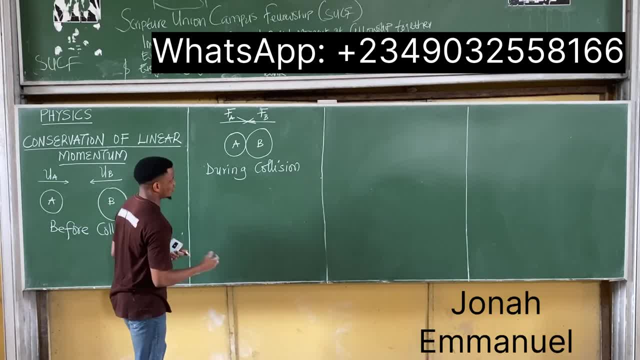 a force, right. So defense, on which direction? all right, You can go in either direction, but for this one, let's assume that they both go in the direction of A. let's say this one and this one, okay, Okay, let's use the size for now. So let's say they both go. 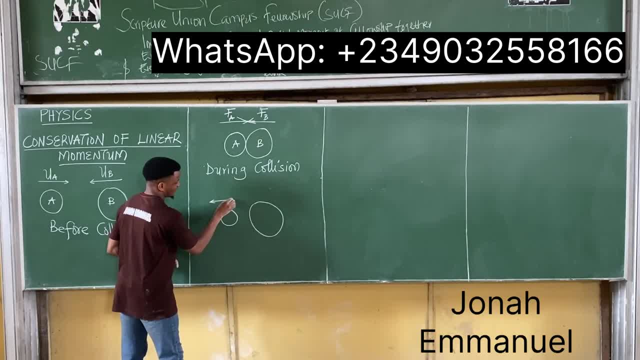 in the direction of B for now. having this Now, this does not mean that objects will always go in the direction of this greater mass or the greater force. no, all right, In some cases can still go in the direction of A. It's possible that they can go this way after collision. 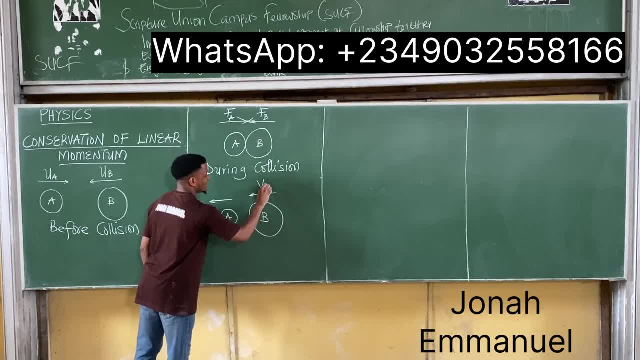 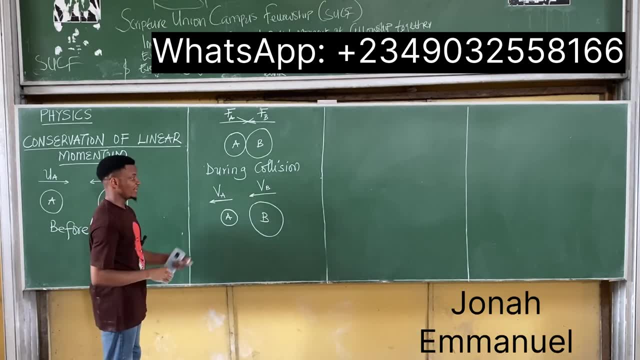 Let me call this V VB- the final velocity after collision. Let me call this VA- final velocity after, or body A after, collision. So I'll call this the after collision diagram. Alright, so you have three diagrams here. This is the diagram, the first diagram here. 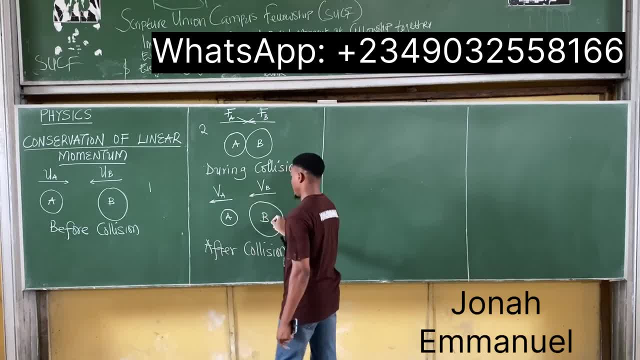 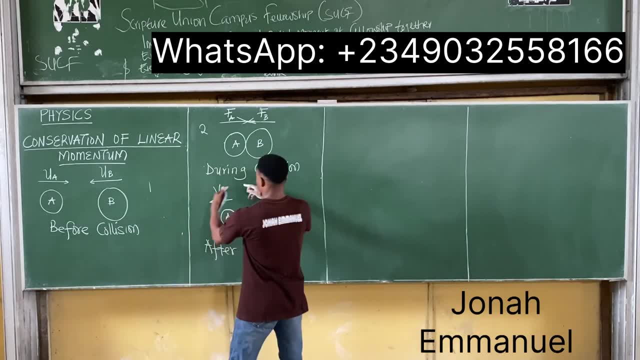 diagram 1.. This is the second diagram. 2. This is the third diagram. 3. Alright, so this is before collision. alright, You are coming in opposite directions. Now, during collision, they hit against themselves with a particular force. Let's now say that the 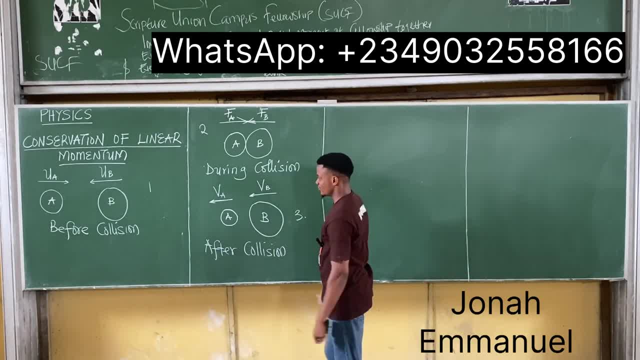 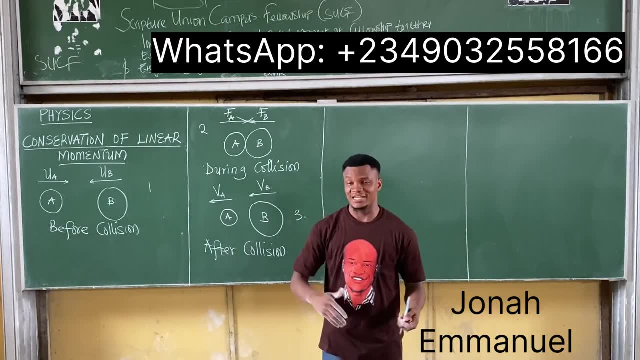 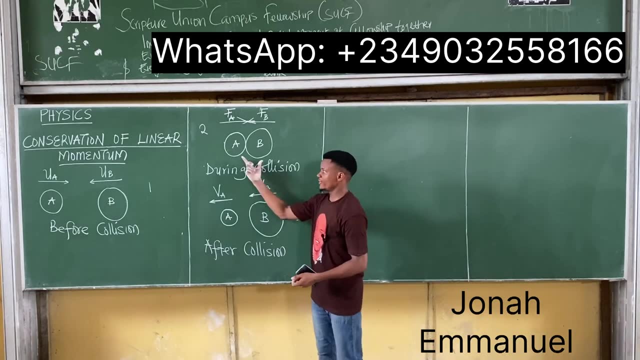 momentum of B is bigger, They will now move in the direction of B. So usually when bodies collide, they will go in the momentum or they move in the direction of the body with the bigger momentum, Not just size. alright, Please think of this. When two bodies collide, both bodies will. 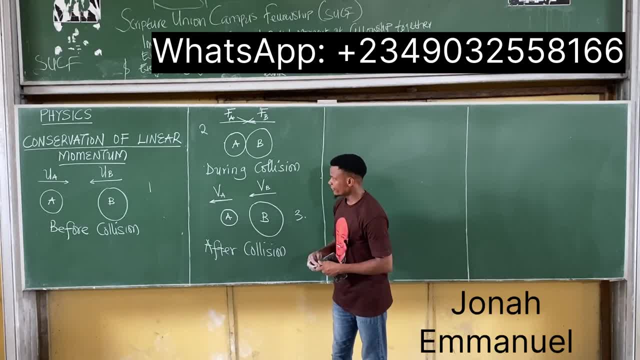 go in the direction of the body with the greater momentum. So for this one here, we are assuming that the one with the bigger momentum is B, Please, momentum is not size. alright, It's not size. So we could have a case where these two collide and they will go in this direction. 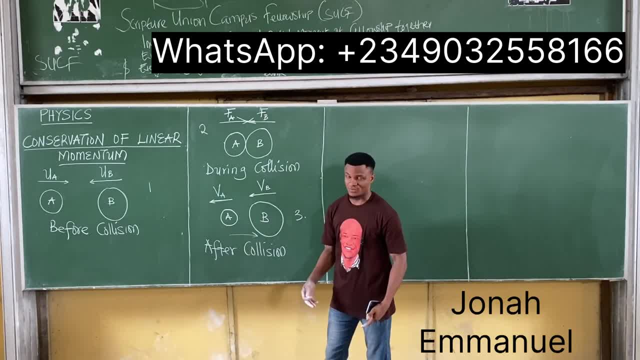 That's this direction. That's, if A has a bigger momentum, they will go in the direction of A. alright, Irrespective of size, Alright. so this is what you should note. So we said that in a system of colliding bodies, that 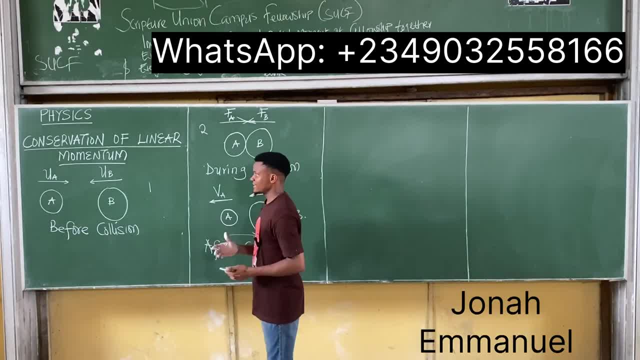 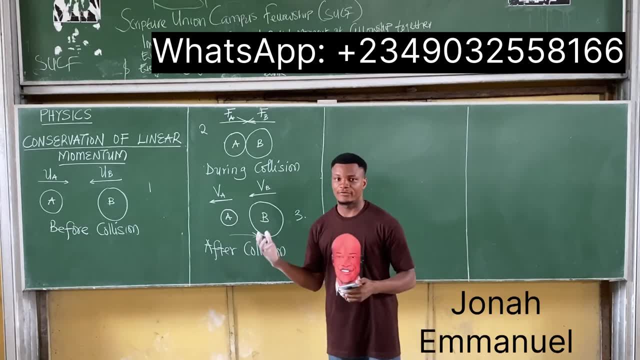 the total momentum is conserved right, Provided that there is no external force acting on the system. Now also, we said something from Newton's third law of motion, which is the law of interaction. We said that to every action there is an equal and opposite reaction. 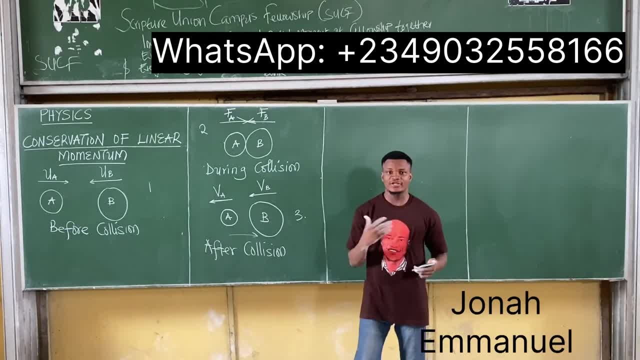 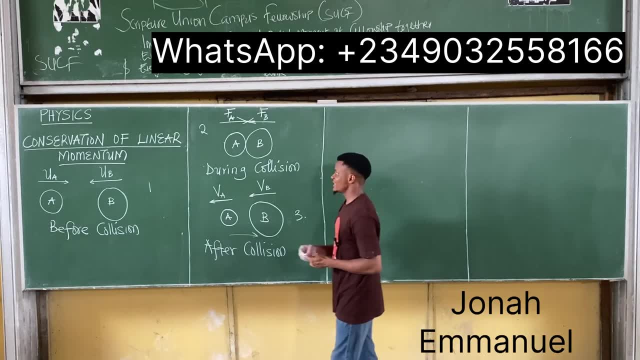 Alright. so if I combine the concept of Newton's third law of motion- which already said is the law of interaction, with the principle of conservation of momentum, it means that if I sum these forces, alright, So this is a system of colliding bodies. We said it would. 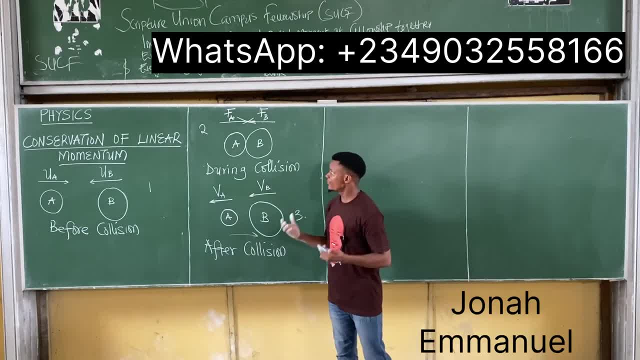 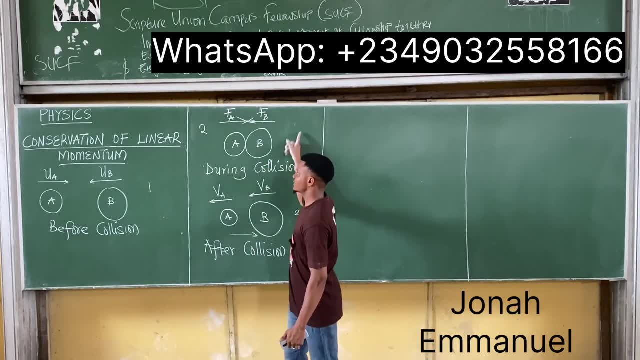 be what Conserved right. So from Newton's third law of motion and from the principle of conservation of an inner momentum, we said for a system of colliding bodies that the total momentum is always conserved Like a constant and constant non- Gateways component. So that means a constant and aian. Create, inamine different models of fighting and playing, So this will result in a way of garden-like structure. So if you solve these…the This will result in a way of garden-like structure. This will result in another project of grandes painting, which 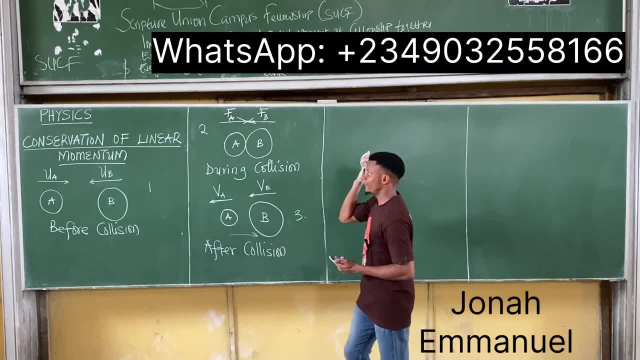 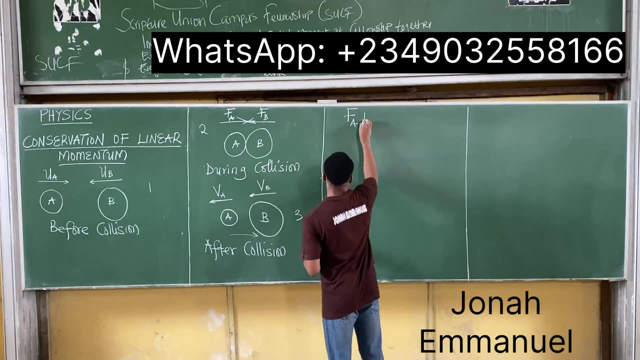 conserved, alright. And in mathematical form we are saying for this case here, during collision, here we are saying that the forces here would be conserved. That means I'm saying that FA, the force with which body A acts plus the force with which body 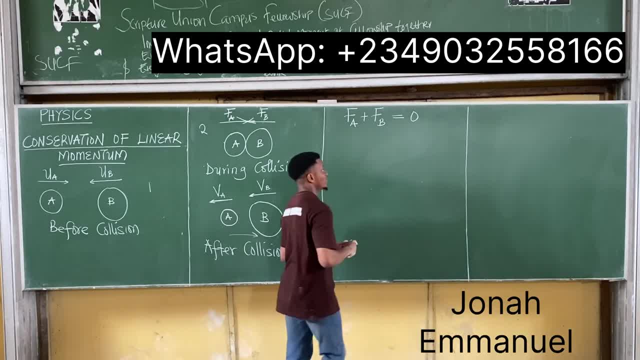 A acts should be equal to zero, alright. So being equal to zero means the net force should be equal to zero because there's no change in force, or there's no change in force because it's a conserved concept, of course for momentum. So I have this. 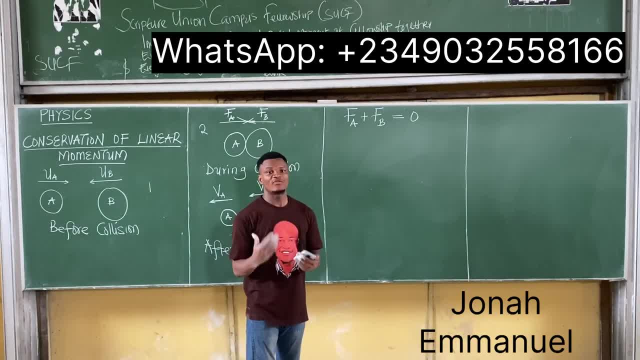 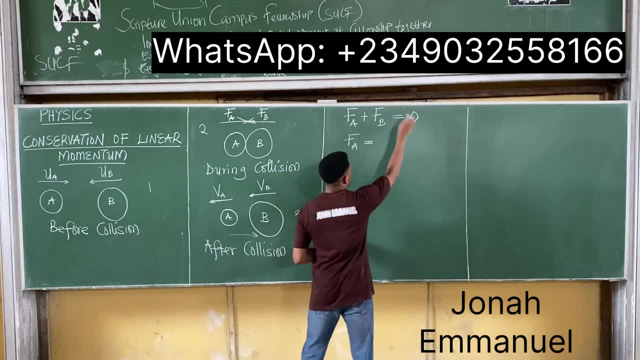 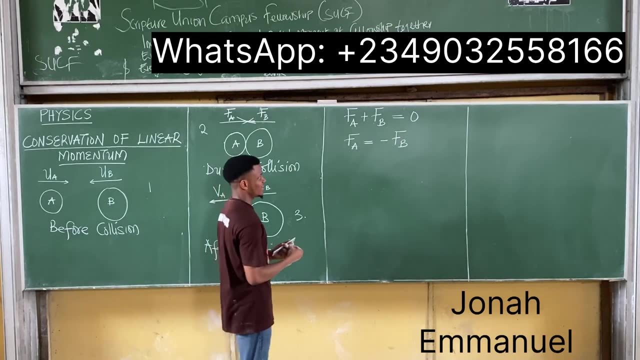 Now, if this is true, record that from Newton's third law of motion- this one goes here and I'll have that- FA will be equal to this. man comes and becomes minus B. So we have this. This is inclined to Newton's third law of motion, which says that to every action, 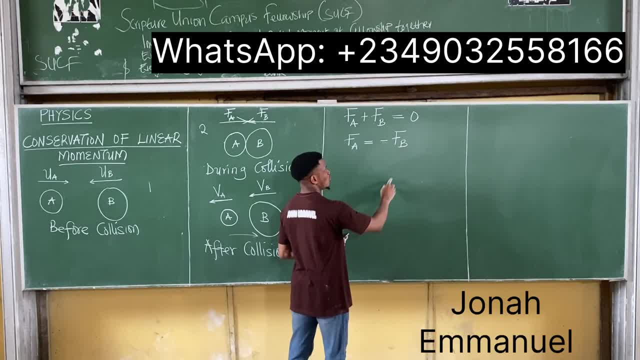 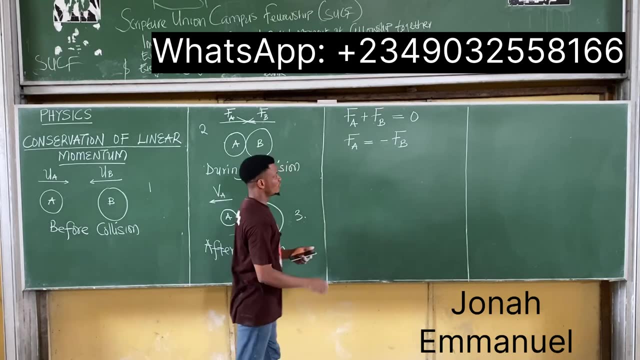 there's an equal and opposite, So negative shows opposite reaction. This is like a mathematical expression of it. To every action, Newton's law of interaction: to every action there's an equal but opposite, Negative showing opposite interaction. This is like Newton's third law of motion. 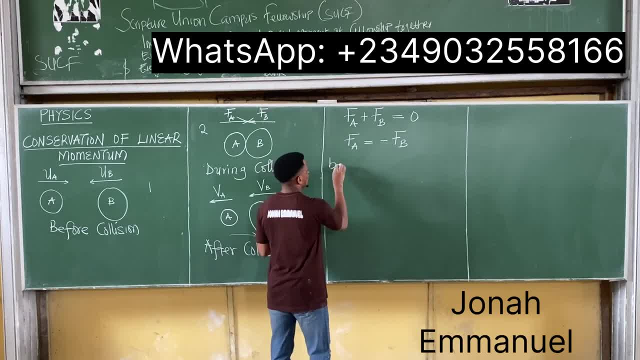 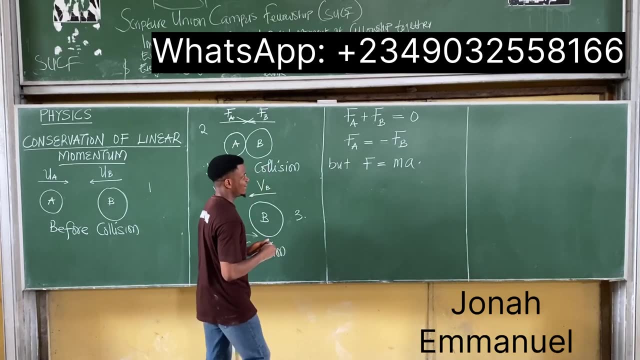 the idea. Okay, but again, but we know that from Newton's second law of motion that F is equal to mass times acceleration. We know this from Newton's second law of motion. Now, if this is true, now what do we have here? It means that 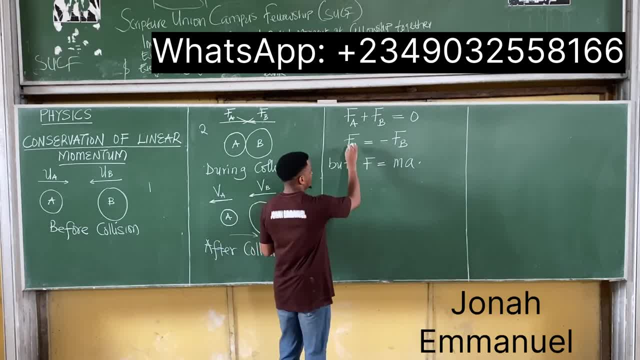 for the first one, FA. it means that for FA we'll have that in place of FA, I'll be having mass of the first one. Now for this one here, observe, we have two different bodies, alright, Body A and body B, So it becomes MA. 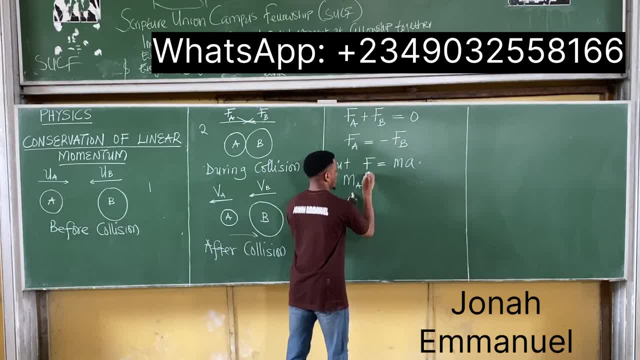 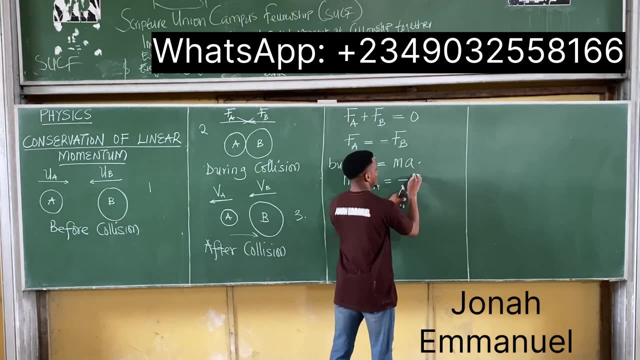 So FA becomes MA, then A AA, Right, Right. The force of A becomes the mass of body A. multiplying the acceleration of body A is equal to negative. the force acting on body B becomes the mass of body B, multiplying the acceleration. 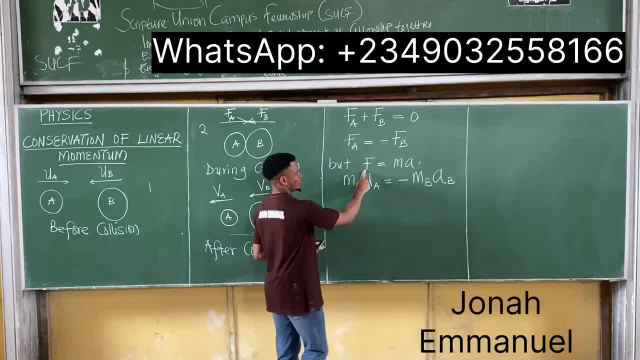 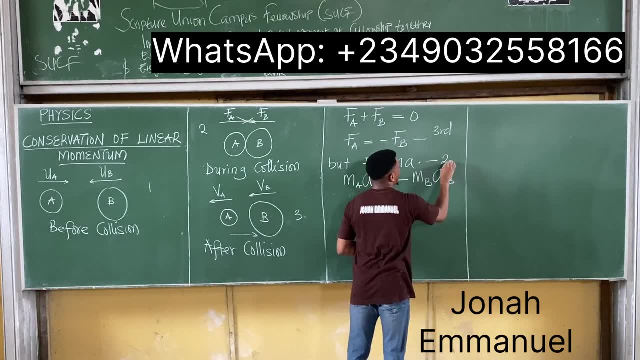 of body B. So I have this right. So F is equal to MA. This one here was from Newton's third law of motion, This here is from Newton's second law of motion. We combine the two concepts and we are here that MA AA. 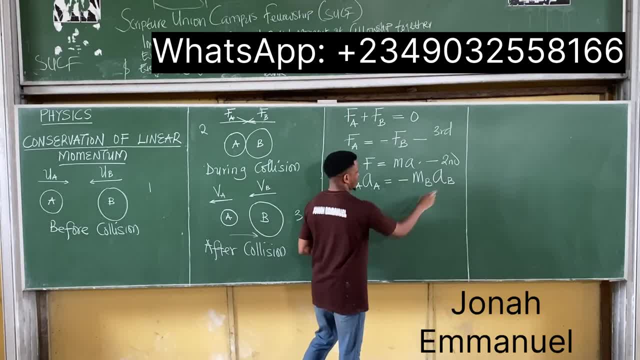 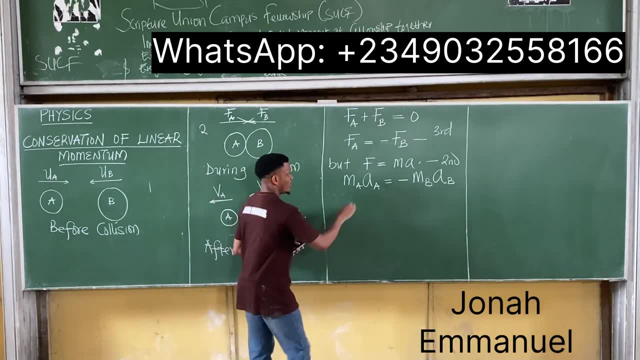 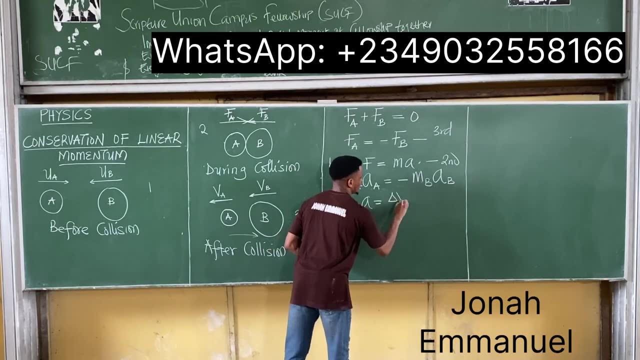 is equal to minus MB AB. Okay, let's bring in other concepts. Now we're talking about the concept of linear momentum. Let's talk about momentum, But again, we know that acceleration A is equal to change in velocity. 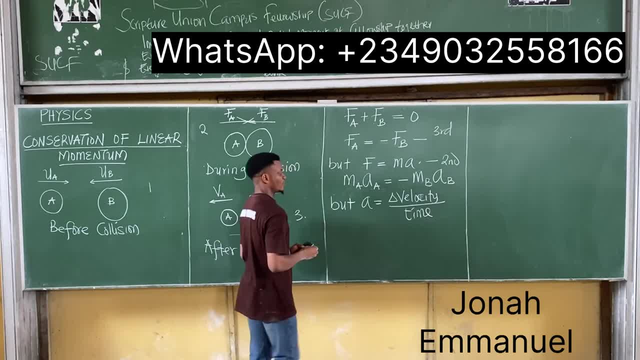 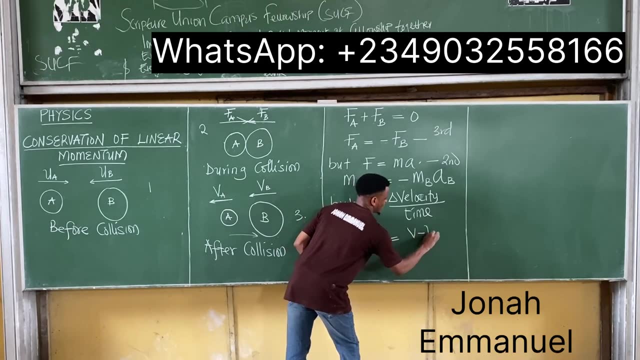 all over time. We have this. So if this is true, that means acceleration A is equal to change in velocity, v all over t, and that's equal to change in velocity, is equal to the difference between final velocity and initial velocity. that's change in velocity. 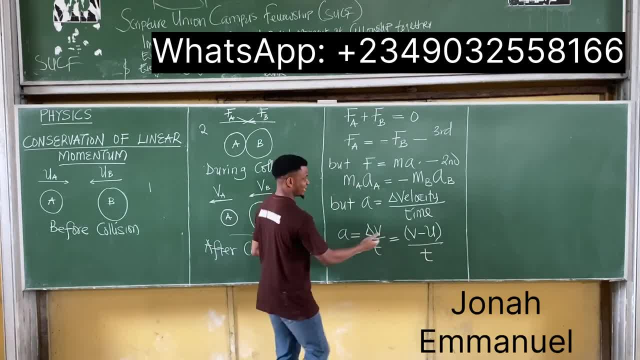 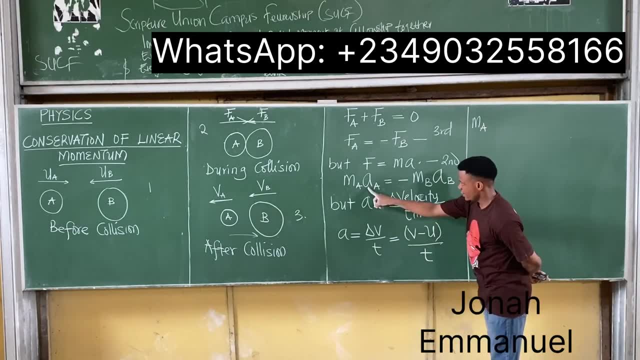 all over time. Now bring this concept here. I will have that m e in place of a e, but we'll just say: a is equal to v minus u all over t For this. here I'll now be having something that looks like this: So, in place of 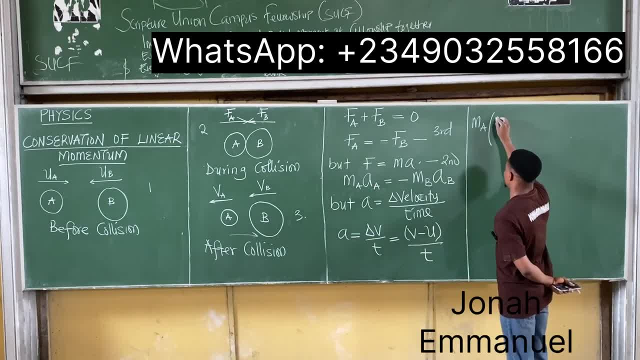 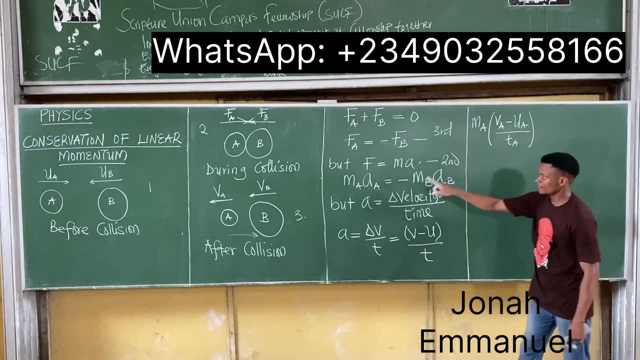 a e. so a is equal to v. it becomes v a minus, u becomes u a all over t. For now let's call it t a. So it's basically the same thing m times a. So in place of this a here, I'll just put 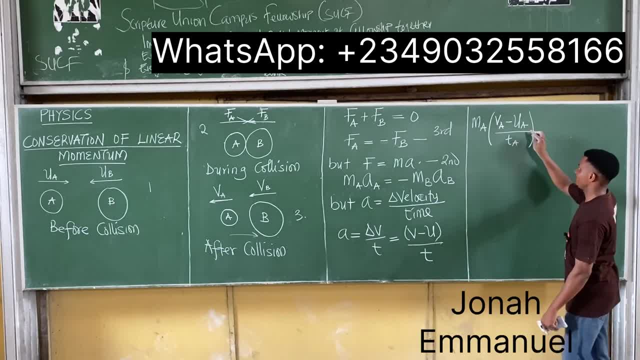 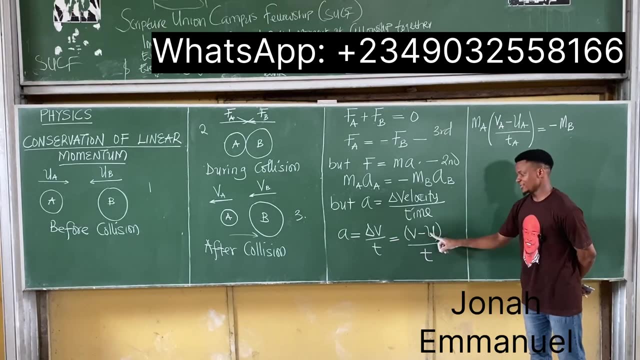 small a, small, a small a. Bring the value of a here is equal to minus. I have minus m b, so minus m b into a, b. Now what's a? We said acceleration is equal to final velocity minus initial all over time. Just attach b to e to the top of this, it becomes. 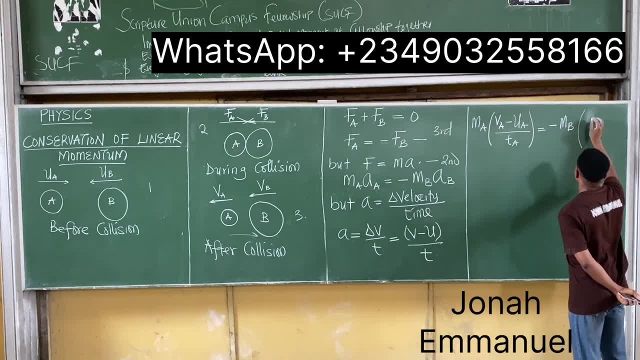 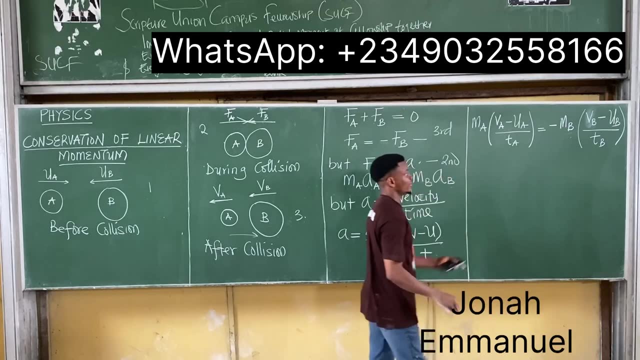 final- sorry, it becomes final- velocity of body b minus u initial velocity of body b all over t time of body b. So we have this Alright. so it's basically the same thing. I'm just putting A and B To differentiate for body A. 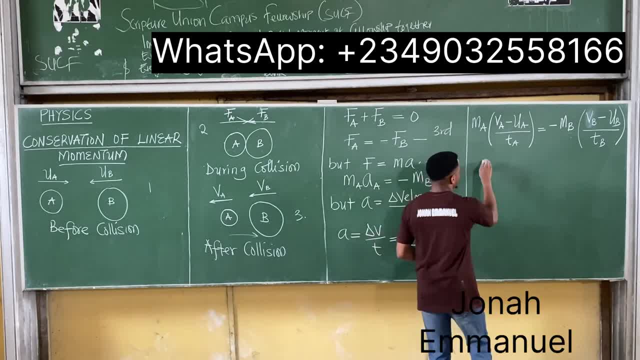 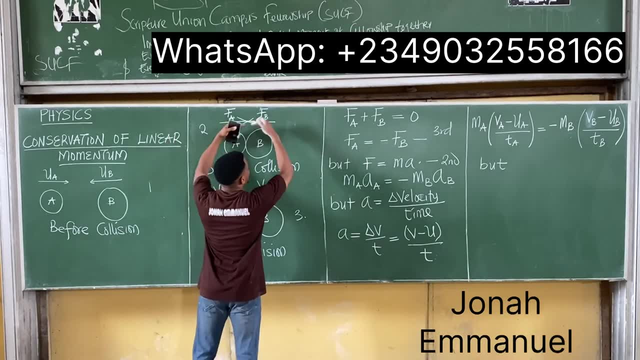 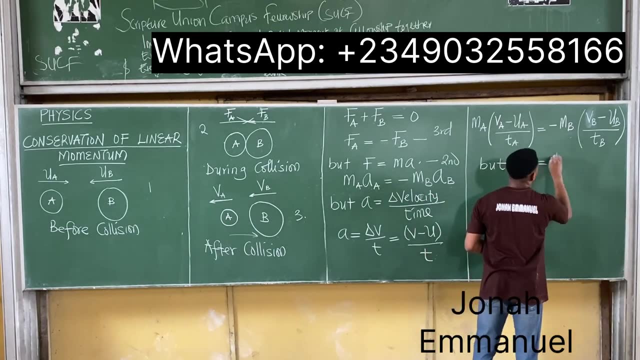 And then body B. But there's something to note. But if you observe, This one here happened at the same time. Both bodies will collide At the same time. If it's collided at the same time, what does it mean? But CA Is equal to CB. Now, this is true. 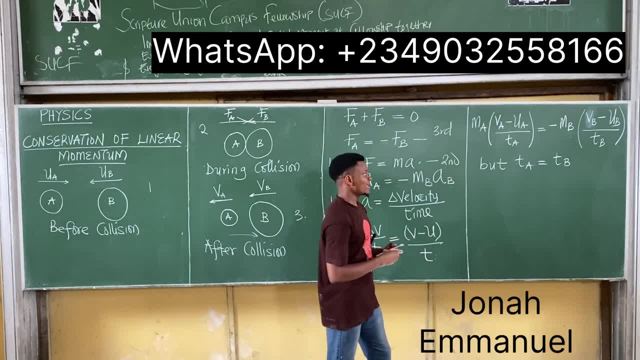 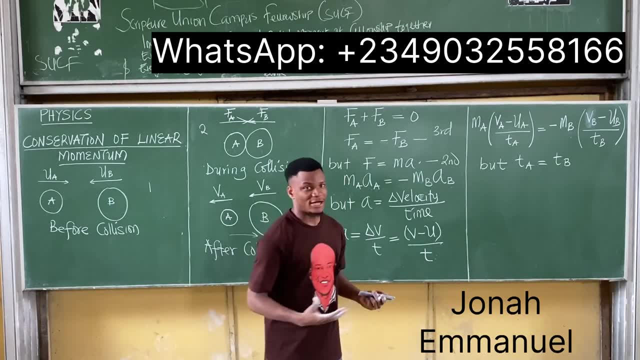 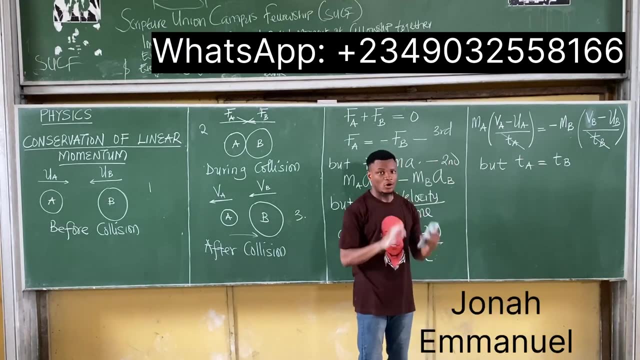 Because the bodies are colliding At the same time. Now, if they are equal, There's a concept in mathematics where, If two denominators are equal on both sides, They cancel out. If they cancel out, what happens? It means that this will cancel this. It's a mathematical correct approach. 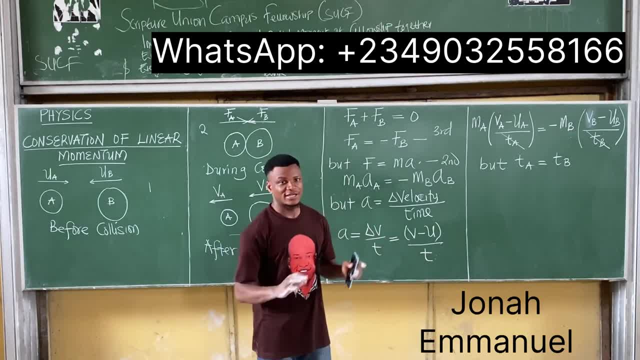 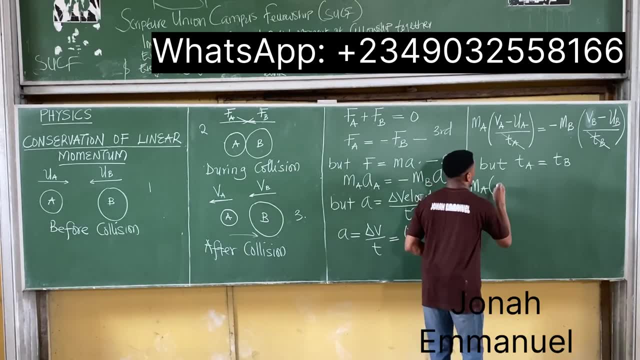 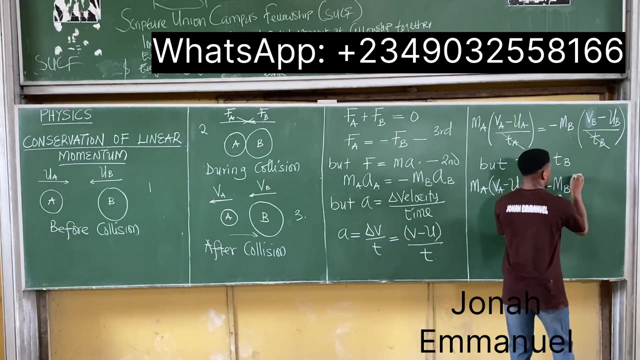 Alright, If two denominators are equal, They can cancel out, and it's correct. So if they cancel out, what do I have? I have just a numerator here Which is MA into VE Minus UE Is equal to this one here Minus MB Into. 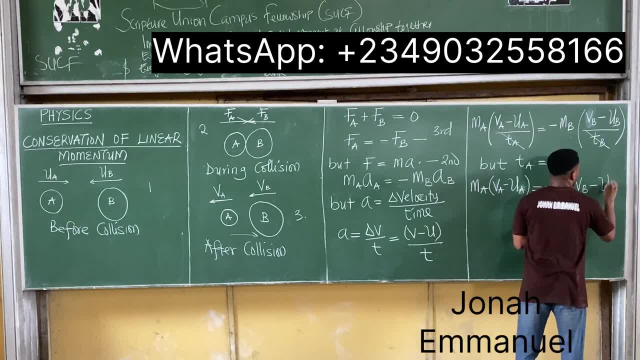 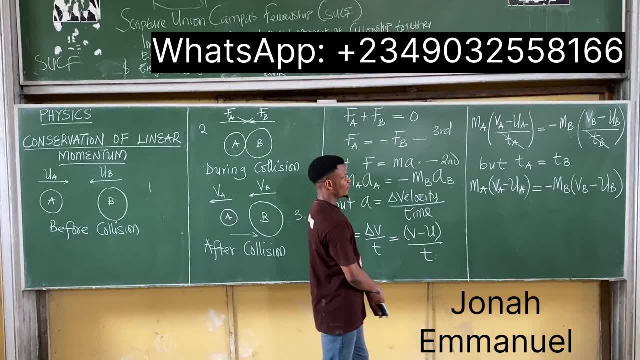 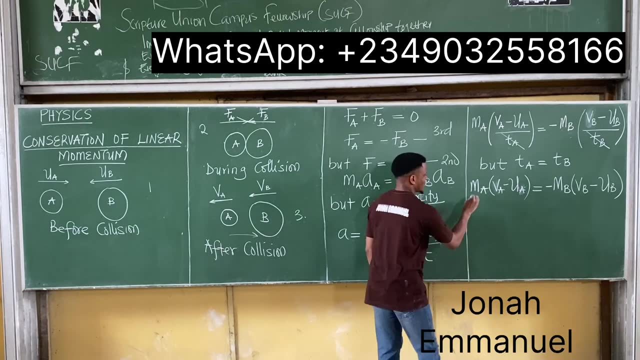 VB Minus UB. So I have this. Alright, so we have this concept here. What next? Of course, denominators are out. My next task would be expanding brackets. So expanding brackets. what do I have here? This and this, I have MA into this. 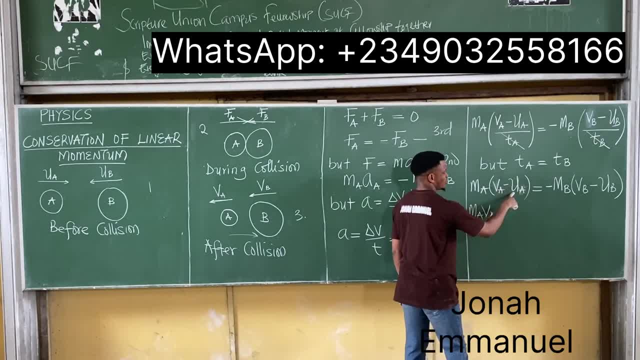 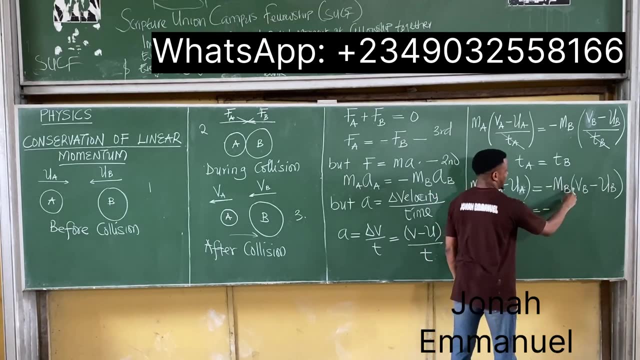 VE This and minus UA Becomes MAUA, The minus sign first. So minus MAUA Is equal to Minus times plus, Minus MB times VB becomes MBVB. Minus times minus Is plus MB times UB becomes MBVB. So we have this, Alright, so we have this concept here. 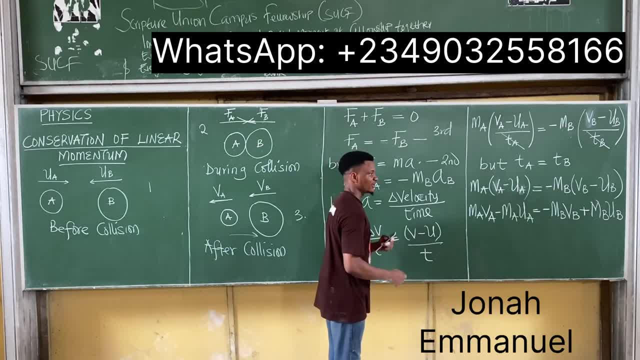 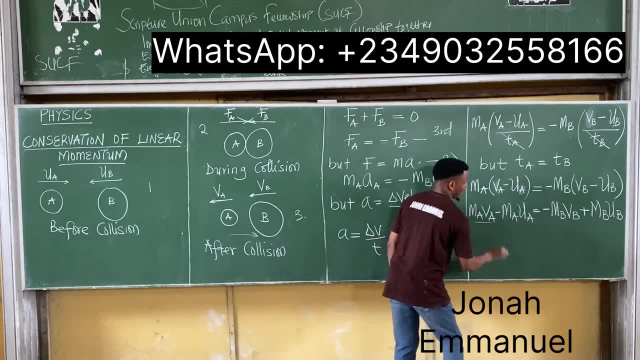 Let's move everything Initial velocity to one side And everything final velocity To the other side. So I have final here, I have final here. Let's bring them together. If I try to bring them together, I'll have something that looks like this: MA This one here VE. 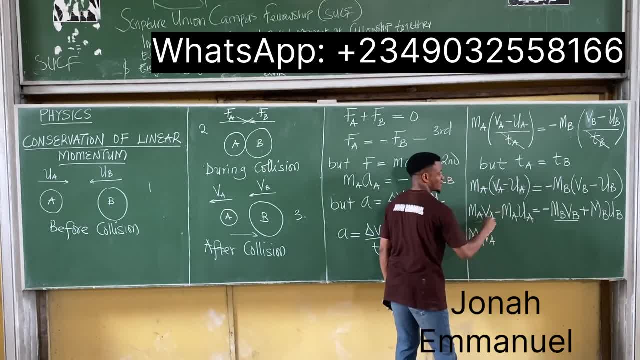 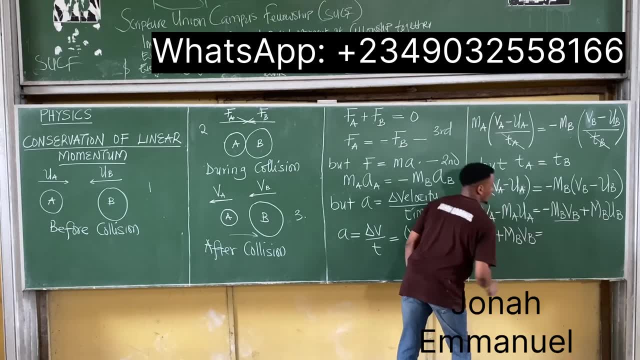 Negative- This is negative- Comes here, becomes positive, So plus. MBVB Is equal to. Let's now move all initials together, Starting with the A. This is negative MAUA- Move it over here. Becomes positive. I'm having positive MAUA. This one is positive, So plus. 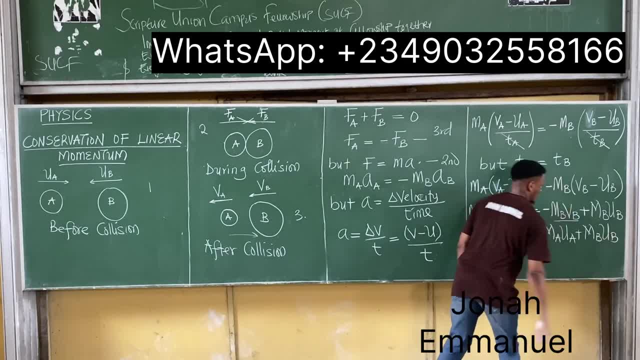 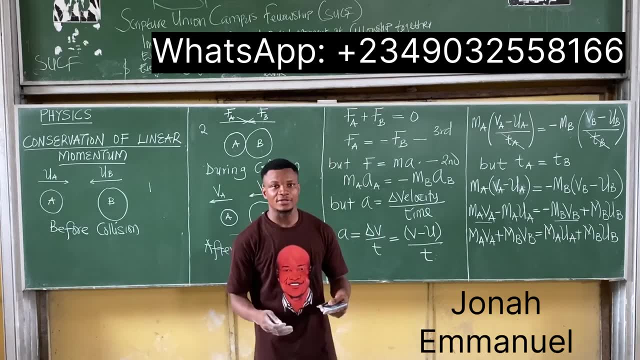 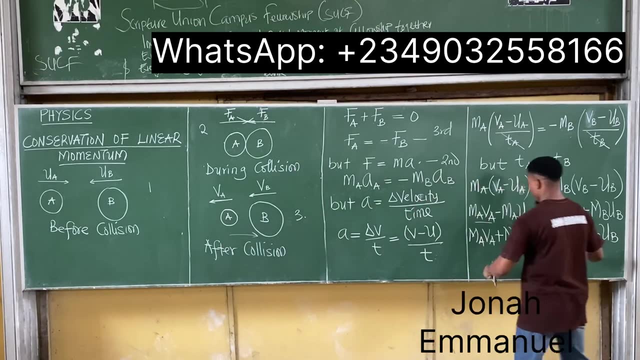 MBVB. So I have this. Alright, so this is what I have. But then, So that we have the A, So that we have the initial Before final, Let's take the initial to the. Let's take the initial to the Left hand side. So move this one over here. 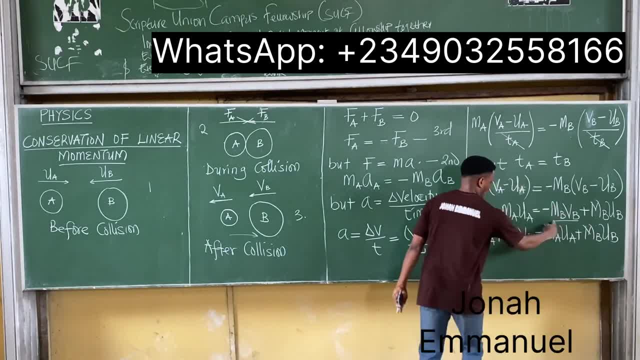 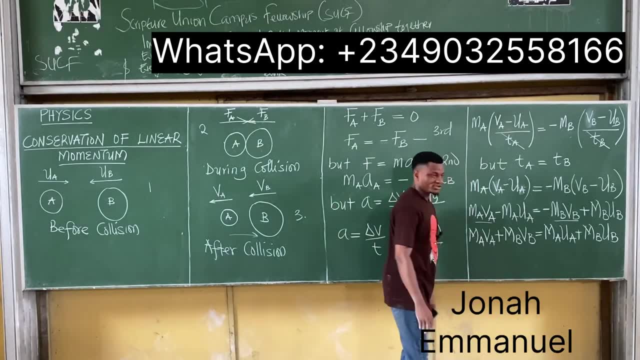 Move this over here. They are the same thing actually. So if I move this one over here, Alright, I'm not actually moving it over, I'm just trying to. Should I use the word reconstruct, Trying to just reconstruct them? Now, I know this one is positive, I know this. 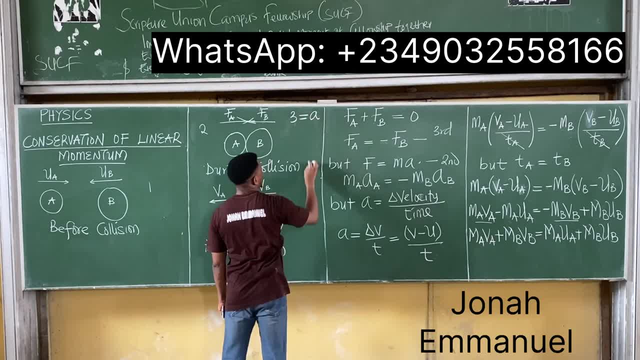 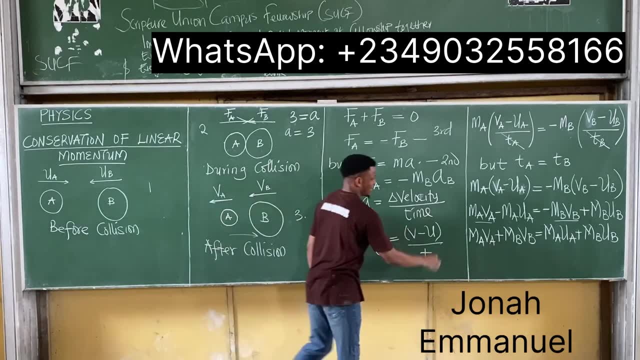 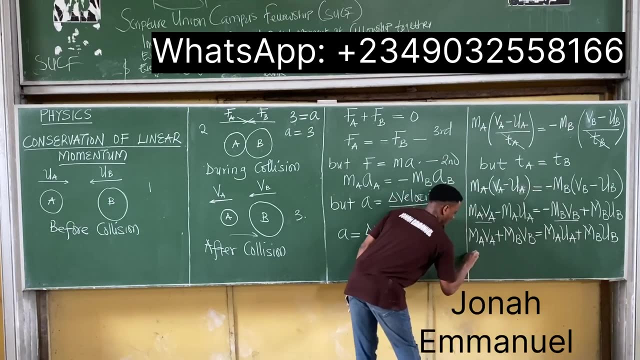 I know that if 3 is equal to A, That means A is equal to 3. I just swapped position And it's correct. Use this idea here. It means that if this is equal to this, Then that means this one here Should be equal to this. That means that. 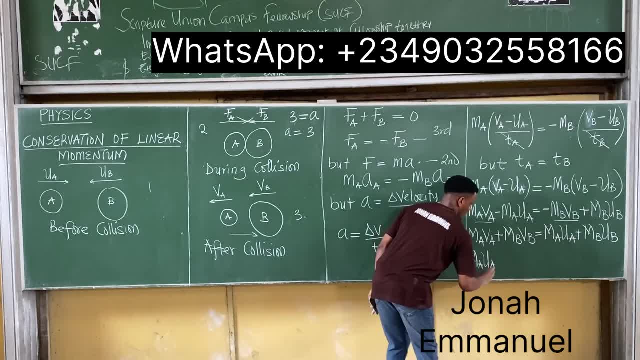 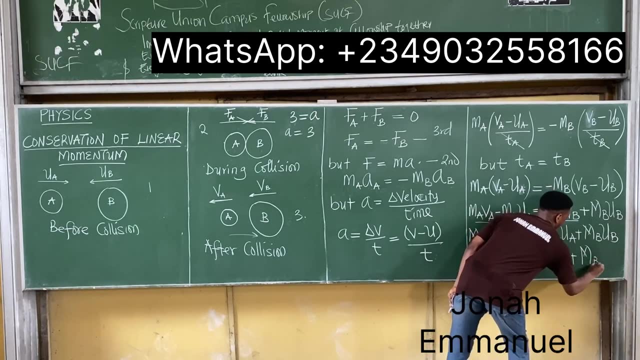 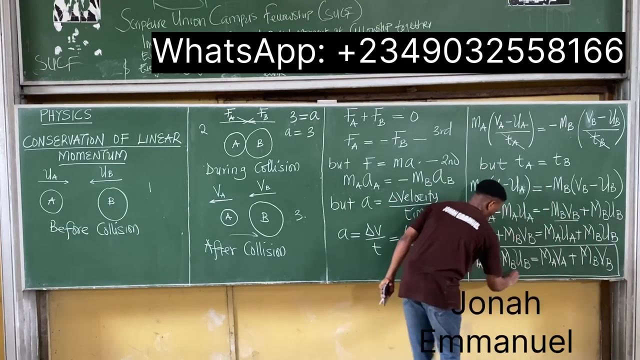 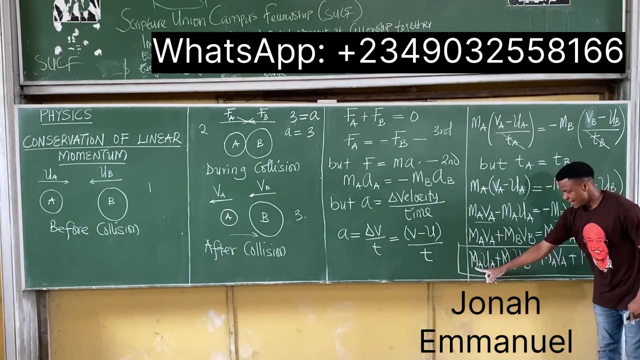 MAUA Plus MBUV Is equal to this one here, That's MAVA Plus MBVB. This becomes the equation For the conservation of linear momentum. Please, This is the equation. Alright, Mathematics. We are saying that The product of the mass And the initial velocity Of the first body 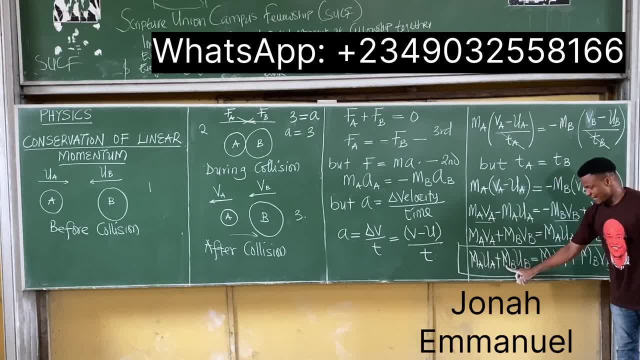 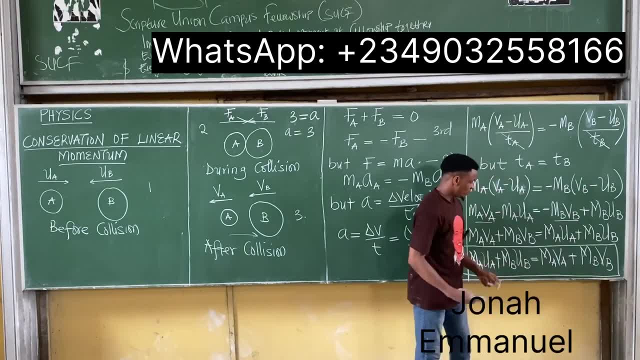 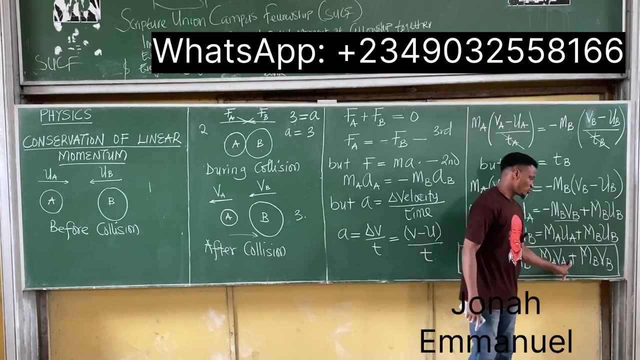 Or body A Plus The product of the mass, And the mass And the initial velocity Of the second body, That's body B, Will be equal to The product of the mass And the final velocity Of the first body Plus The product of the mass And the final velocity. 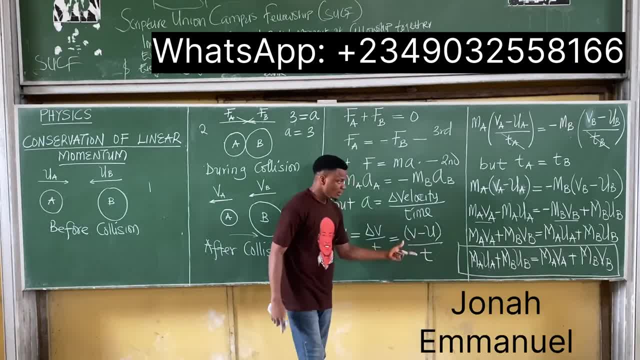 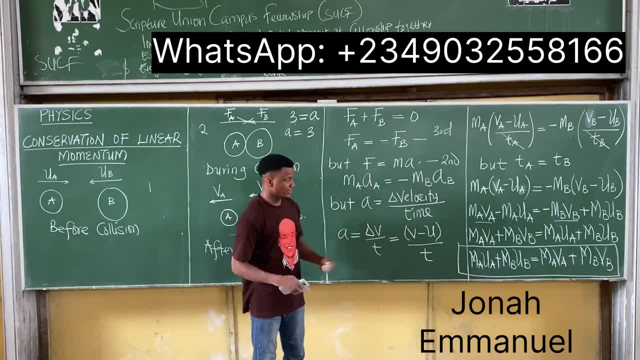 Of the second body. Alright, So this is the Law of conservation of linear momentum In mathematical form. Alright, Let's take some problems on this And then We'll see how we can solve problems On the law of linear momentum in mathematical form. The law of conservation of linear momentum. 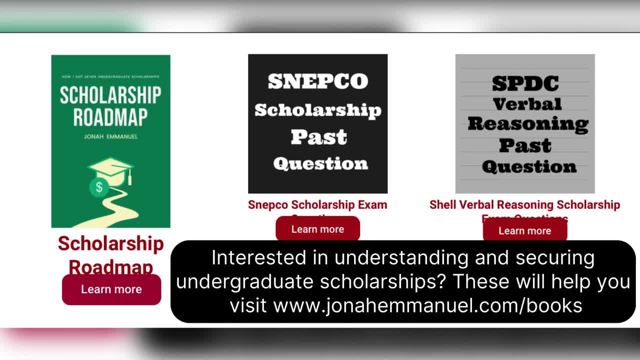 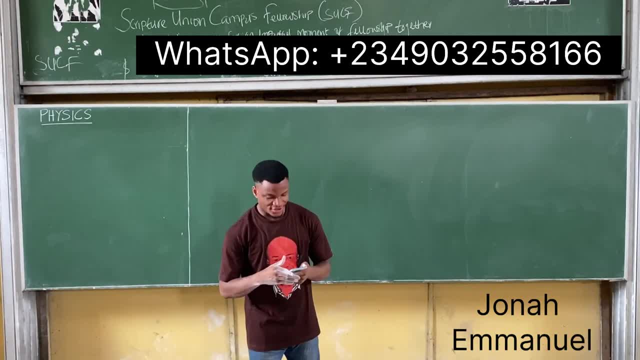 Alright, Let's look at this question. This question says A body of mass- 2 kilogram Moves with an initial velocity 5 meter per second And collides with another body of mass- 15 kilogram- Moving at 0.3 meter per second. 0.3 meter per second. 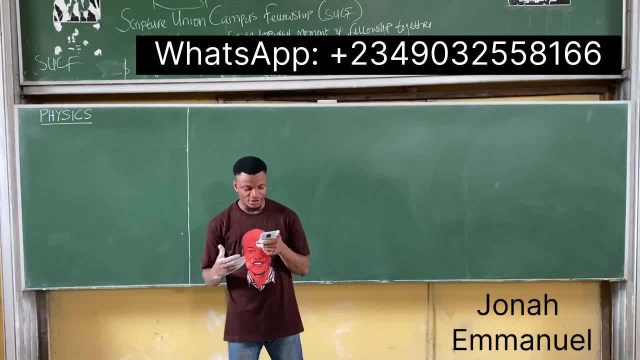 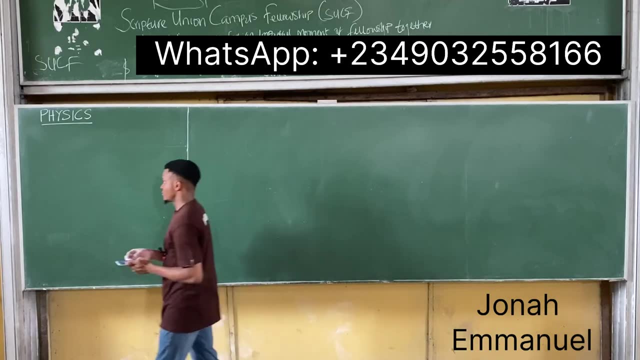 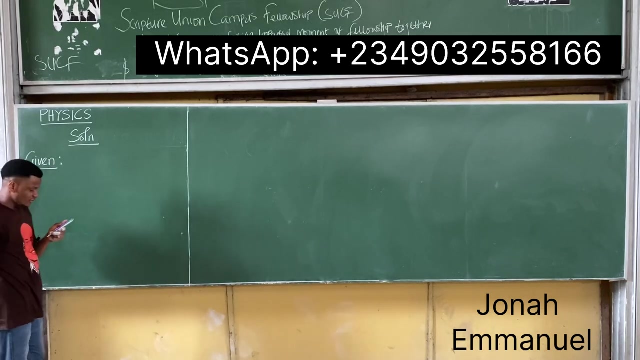 full stop. if, after collision, the body of mass two kilogram moves with a velocity of four meter per second, what is the velocity of the 15 kilogram body? all right, let's get this done, please. so solution: solution given, given. let's list our given parameters: solution by one. they said a body of mass two. 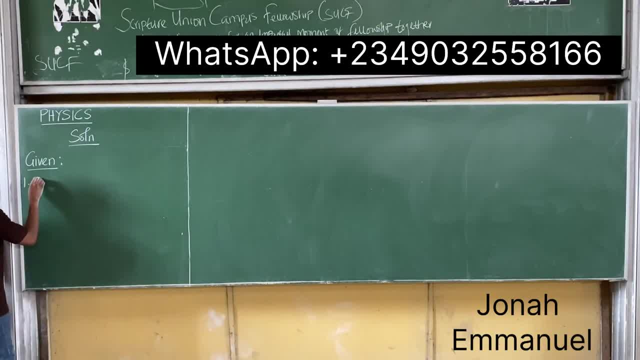 kilogram. so let's call this body one or body a body body one or body a. let's say mass of a is equal to two kilogram. okay, they said moves with an initial velocity about two. I have the initial velocity of this body, a, as equal. 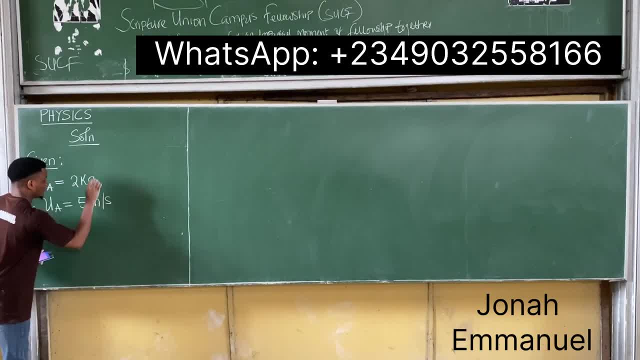 to five meter per second, per second, okay. next episode, and collide with another body of mass, 15 kilogram number next up. I'm giving the second mass, so let's say MB, as equal to 15 kilogram. moving at 0.3 meter per second by 4. it means that the initial 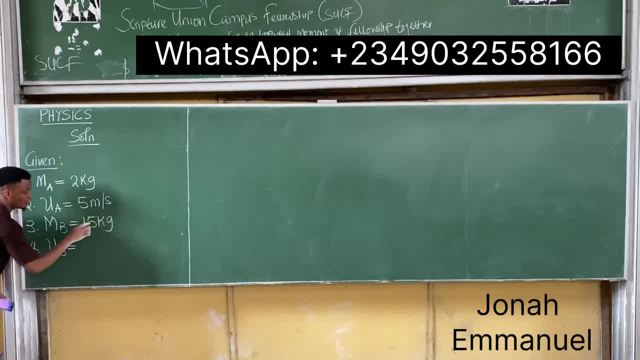 velocity of this second body B or of the 15 kilogram mass. so the initial velocity of this second body B or of the 15 kilogram mass body is about 0.3 meter per second. what's next there, they said, if after collision the body of 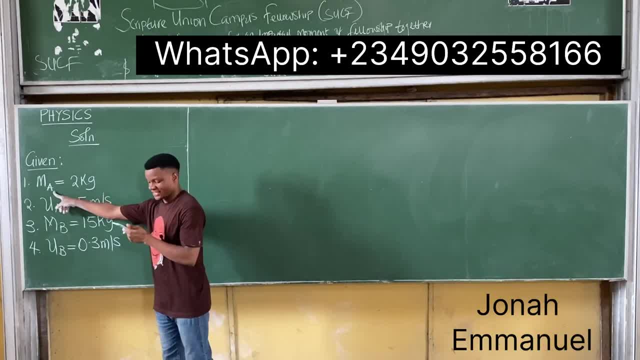 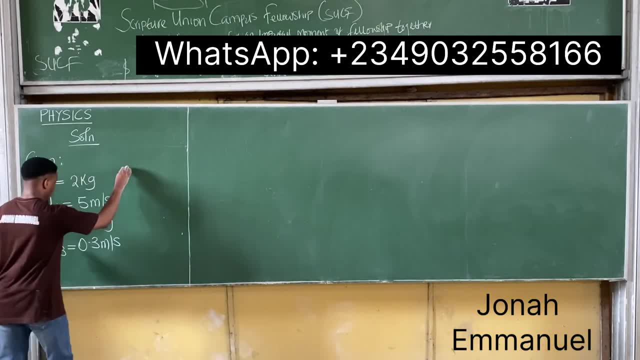 mass 2 kg. the body of mass 2 kg is the first body they said- moves with a velocity of 4 meter per second. that means the final velocity. let me call this 50 on there. that means v by 5, v of a is equal. 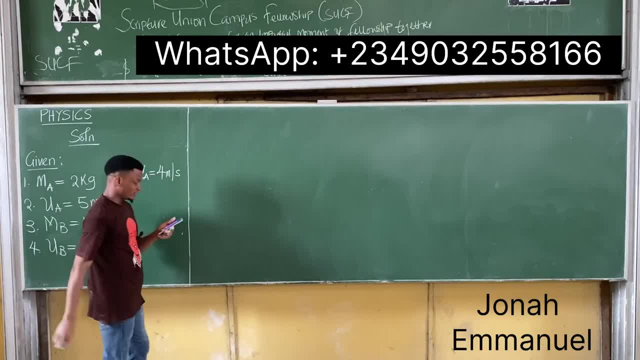 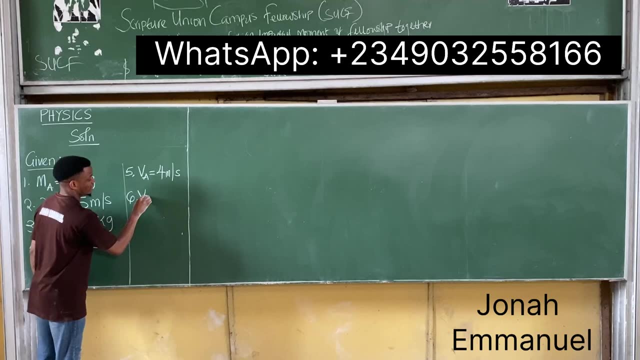 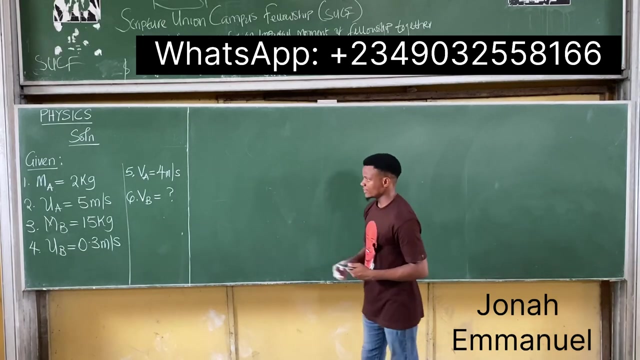 to 4 meter per second. okay, what is the velocity of final velocity of the 15 kilogram um body? that's this one. here we have to find v. final velocity of b is equal to unknown. all right, we have to find this. so quite a simple question from here. let's recall. let's recall the equation. 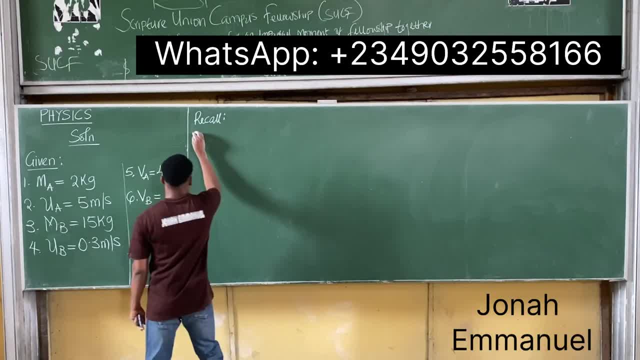 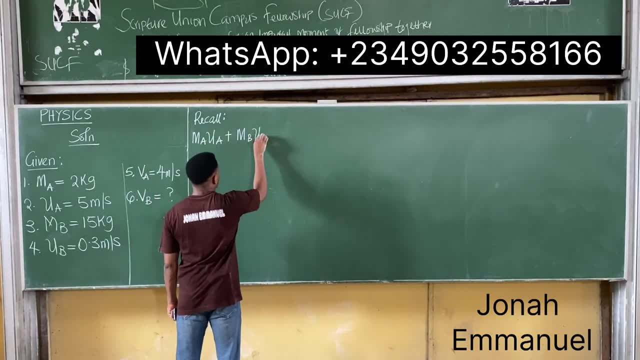 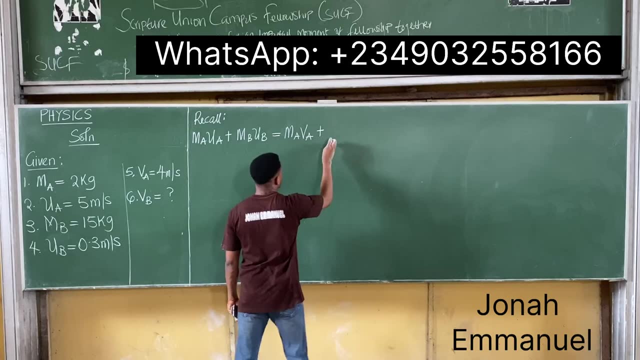 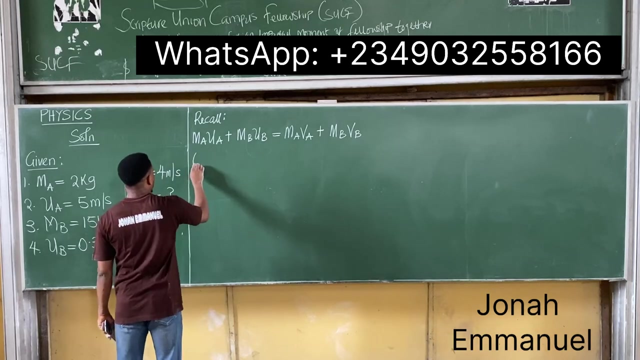 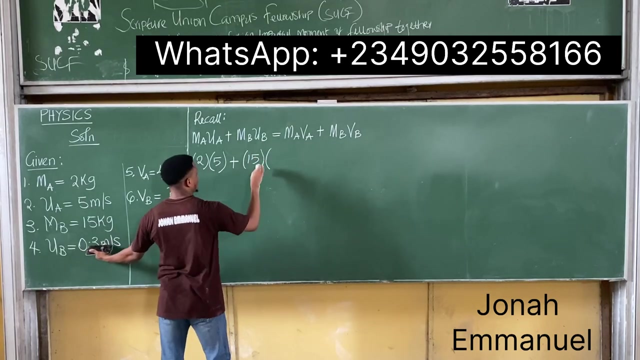 of conservation of momentum. it says that m a- u a plus m b u b is equal to m a v a plus m b v b. all right, bring in values. m a is about 2 into u. a is about 5 plus m b, that's 15. 15 into u b, u b is about 0.3. okay, is equal to. now i am imputing the values. 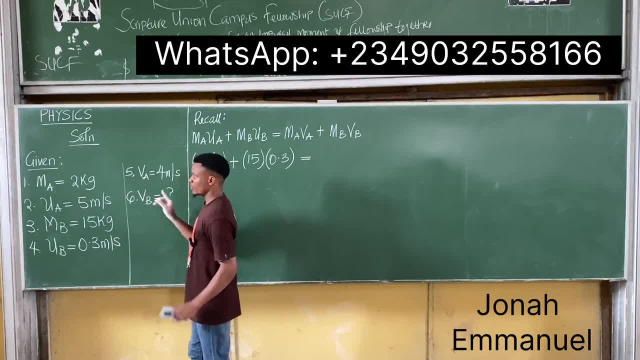 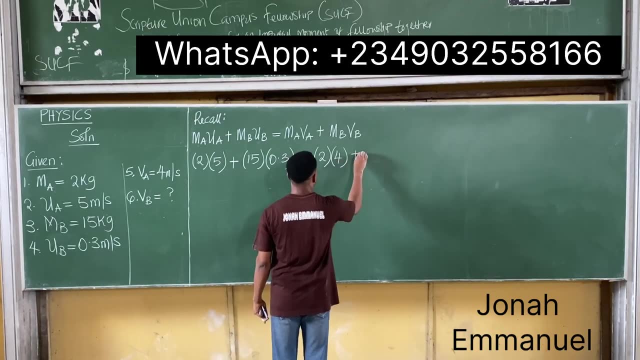 because all the s? i units are in their basic form, so i'm not converting. all right, um m a again, m a is 2, that becomes 2, into v a. v a is 4, that becomes 4 plus m b. uh, m b is about 15 becomes 15 into v b. that's the unknown. 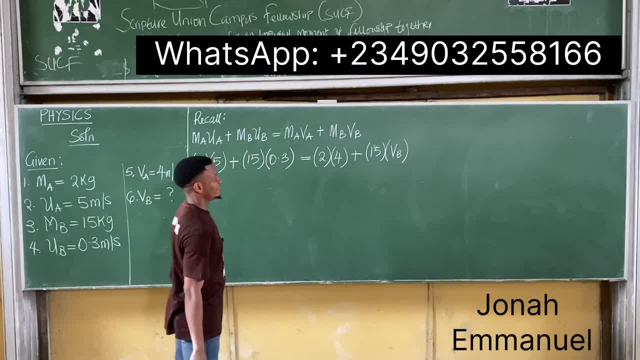 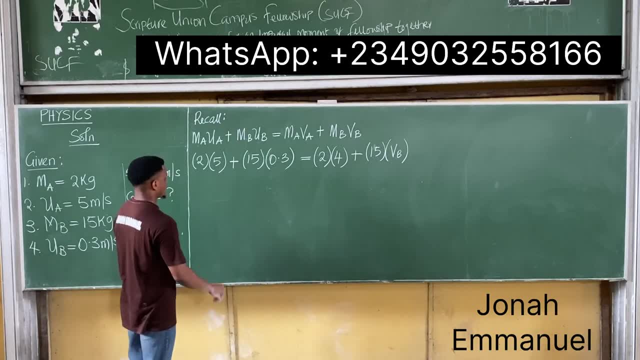 value which we have to find the final velocity of the 15 kilogram mass or body. all right, so let's multiply this. so first things first, we have 2 times 5, that's 15 plus 0.3 times this, that should be about 4.5. so 4.5 15 times 0.3, that should be 4.5. 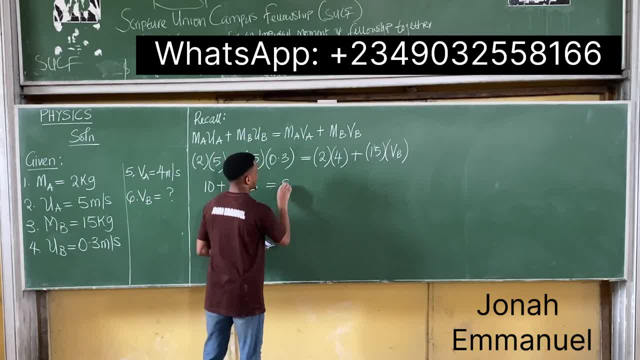 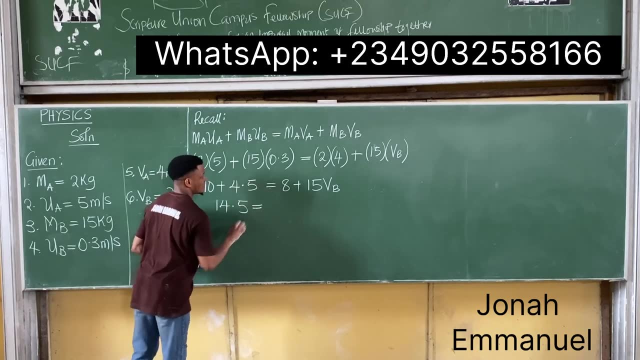 okay, is equal to 2 times 4, that's 8 plus 15 times vb 15. So I have this. 10 plus 4.5 gives you 14.5 is equal to 8 plus 15 VB. So I have this. 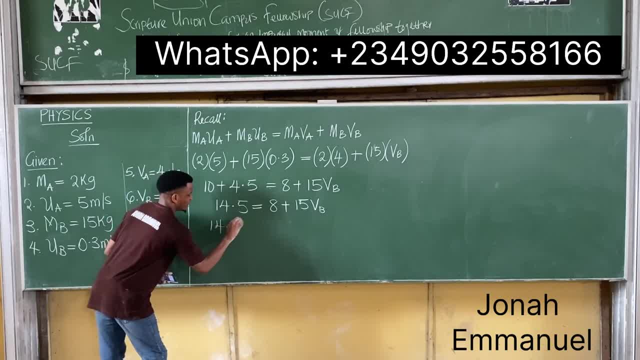 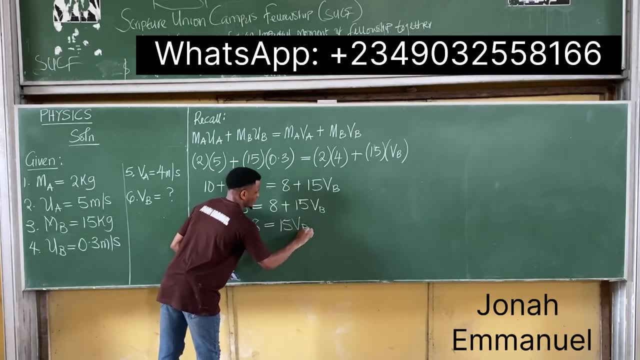 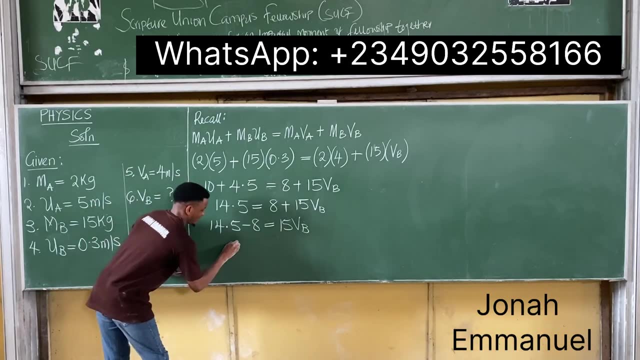 So move this one over here. 14.5, 8 comes and becomes minus 8 is equal to 15 VB. I'll do a little subtraction: 14.5 minus 8 is about 6.5.. So 6.5 is equal to 15 VB. 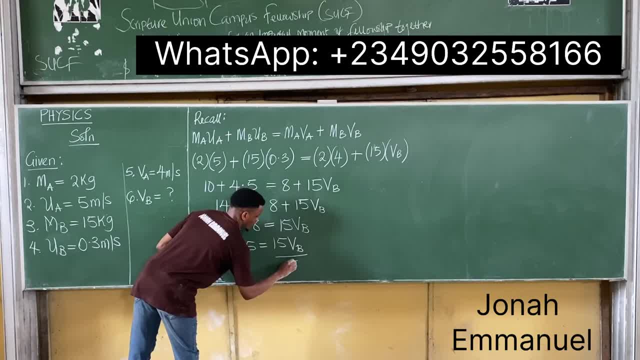 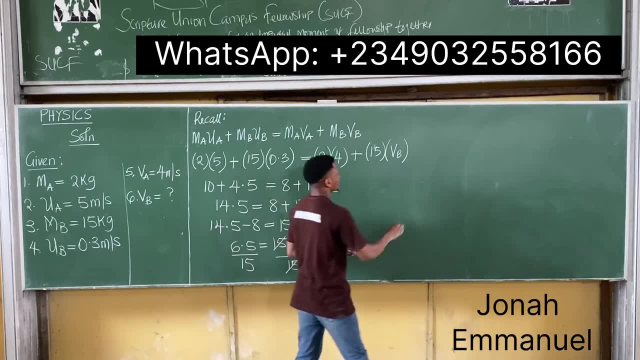 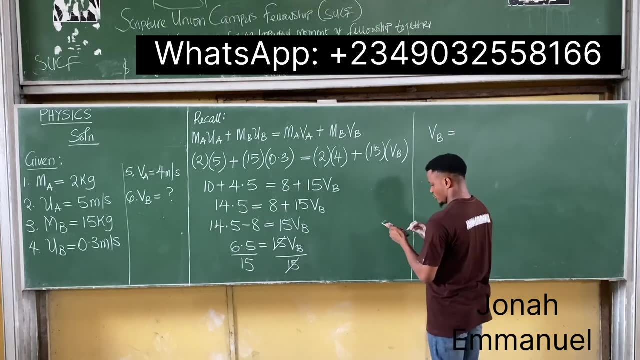 So against VB. I'll divide here by 15.. I'll divide here by 15.. This cancels this, So, VB, I'll have that. The final velocity of the 15 kg body is equal to: so 6.5 over 15, that's about 0.43 in meter per second. 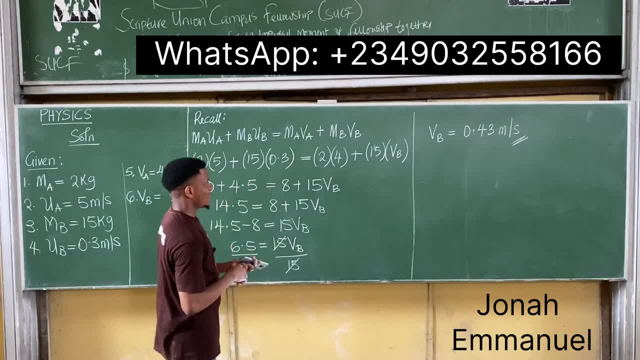 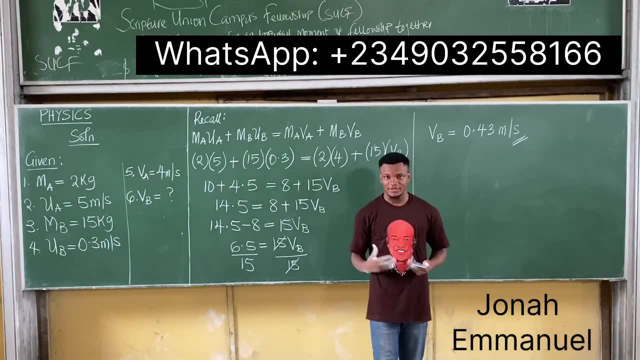 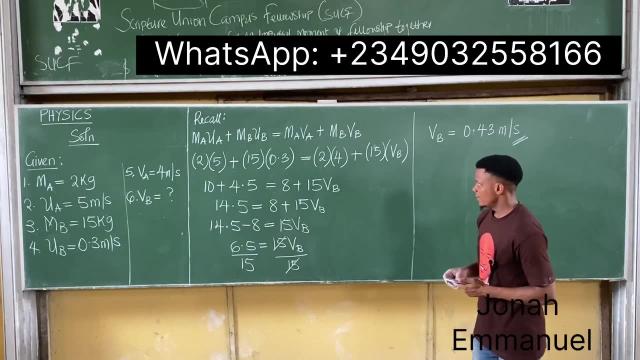 This becomes the answer. All right, This is how I solve this question. All right, So this is the answer to this question. All right, Before we go, let's consider something. Let's try to do a diagrammatic representation of this. 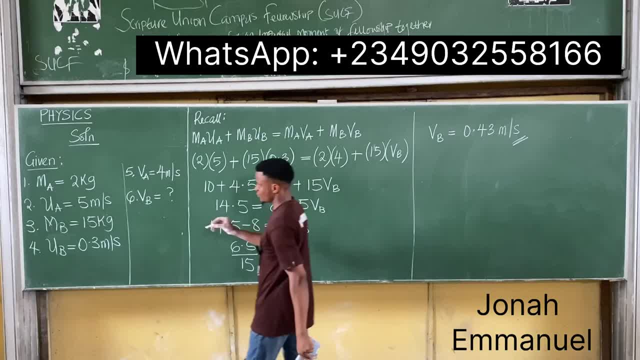 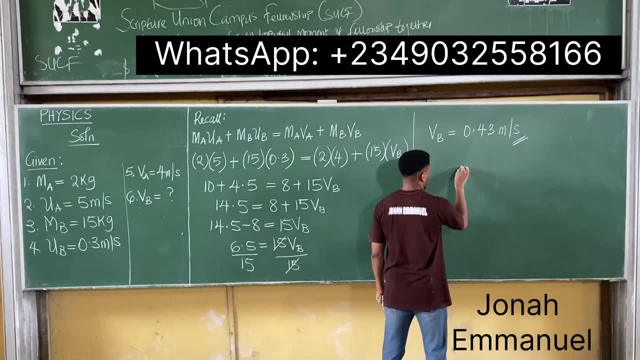 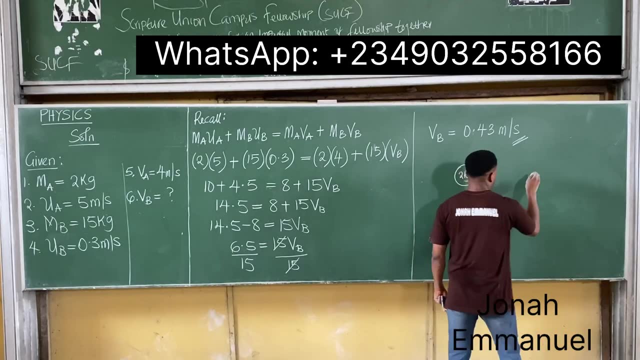 So you have two bodies. The first one is 2 kg, The second one is 15 kg. That means mass A will be smaller per se. Let's just make it smaller. So this is 2 kg mass. Then we have the 15 kg mass. this one here about 15 kg. 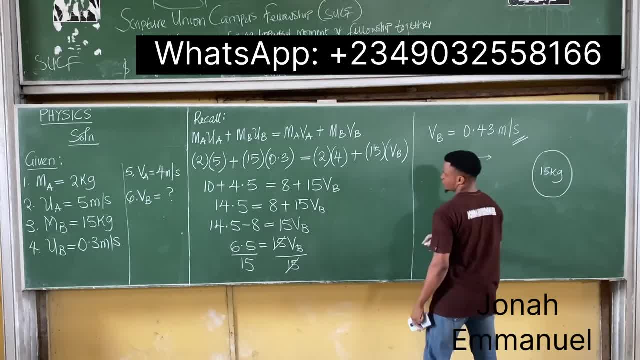 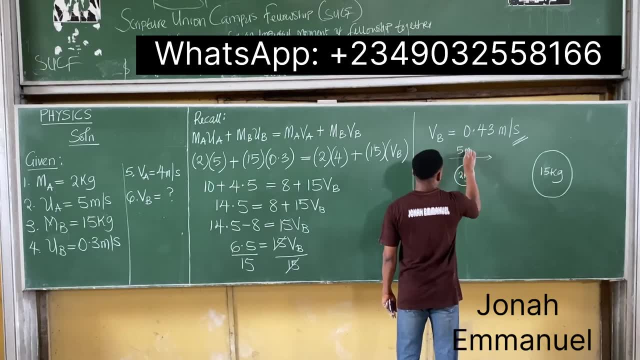 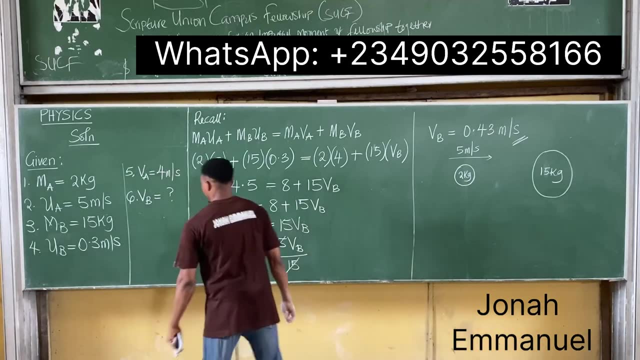 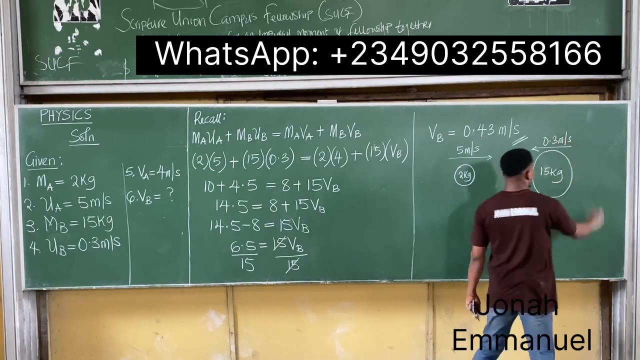 This is moving with a velocity of 2 kg. The 15 kg moves with an initial velocity of 5 meter per second. This is 5 meters per second. The 15 kg moves with initially 0.3.. I'm having this 0.3 meter per second Now. we said these two bodies collided. 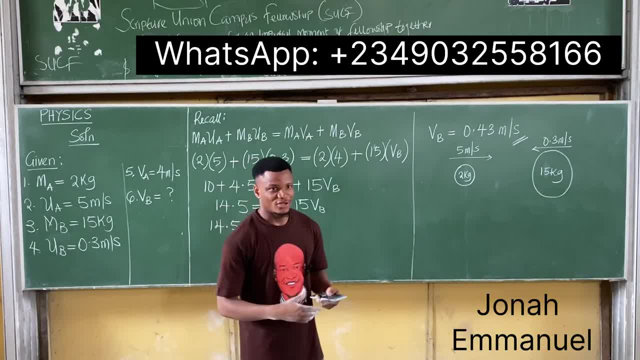 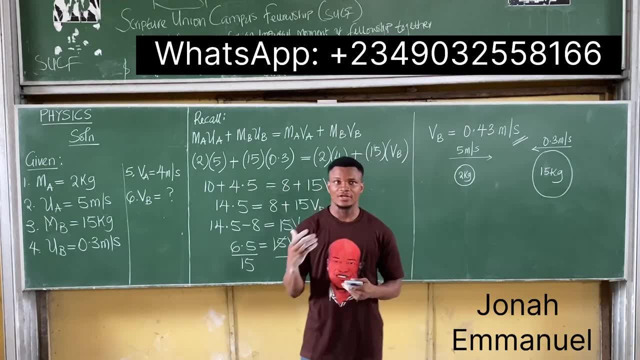 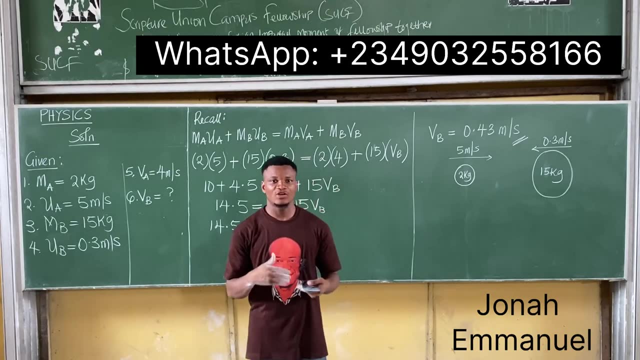 Question will now be: what if you're asked to find the direction that the body moves? So what would you do Now? basically, the direction of the bodies after impact basically is dependent on the direction of the body with the greater momentum. 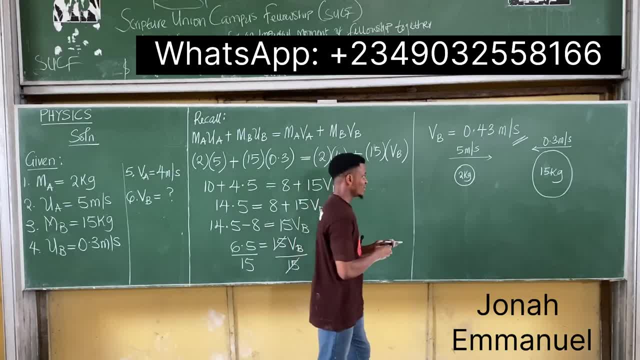 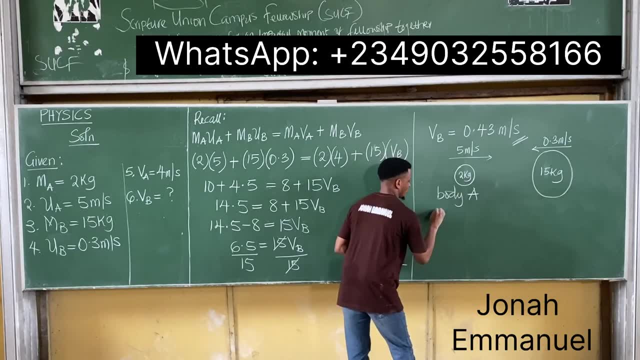 So the question is this: Which of these two has a greater momentum? Let's start with this one. This is body A For body A for body A. here the momentum P is equal to the mass of A times initial of A. 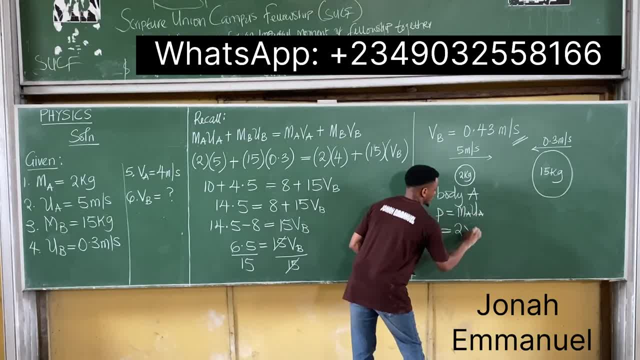 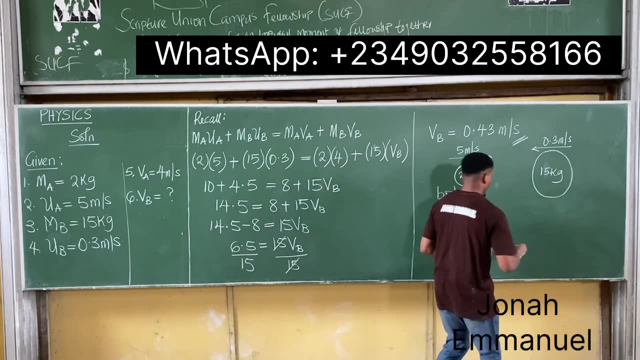 And that's equal to mass of A is 2 times initial velocity of A is 5.. That means body A is moving with a momentum of about 10 kg meter per second. So we have this. Okay, What about body B? Let me call this P A. 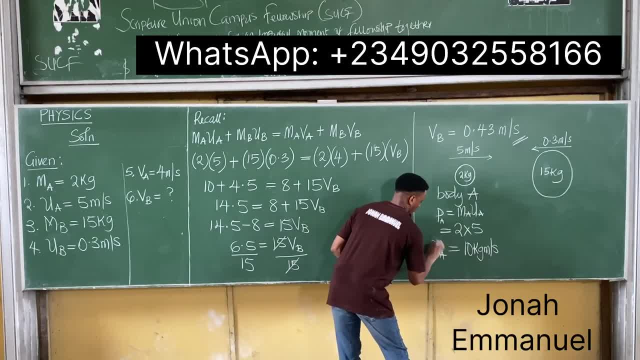 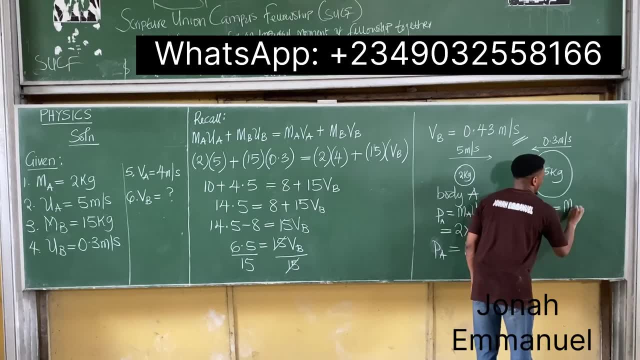 Okay, So P A is this, Because it's small P P A. Alright, Let's come to body B. So the momentum of body B is equal to mass. Mass of body B times initial velocity of body B, And that's equal to what's the mass of B. 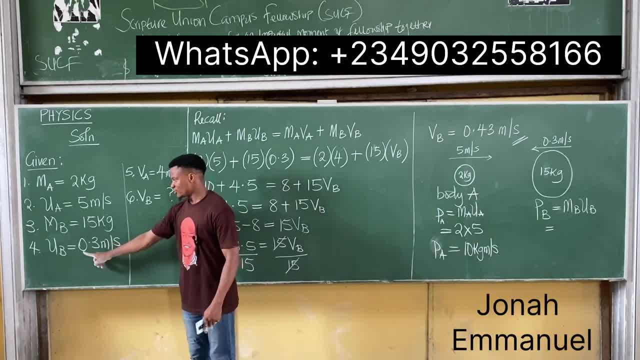 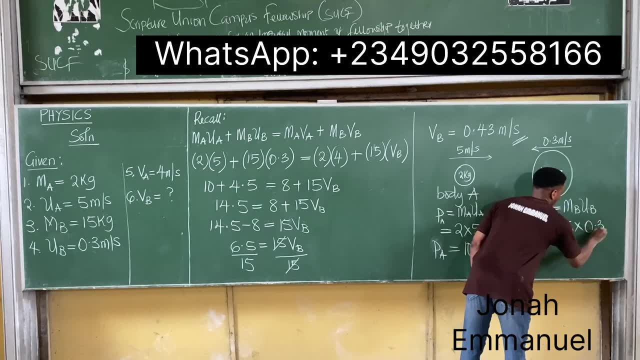 Mass of B is about 15 kg. Initial velocity of B is 0.3.. That becomes 15 times. This becomes 15 times. This is 0.3.. Combine this. This gives you 4.5 kg meter per second. 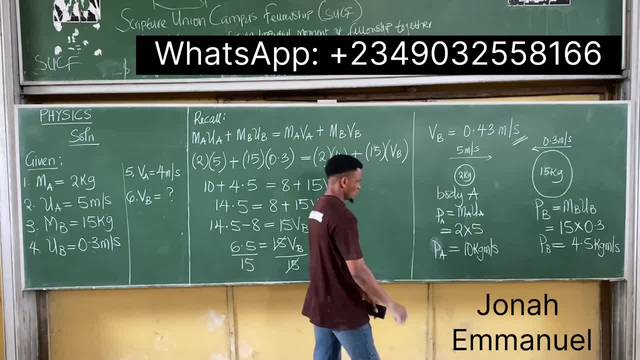 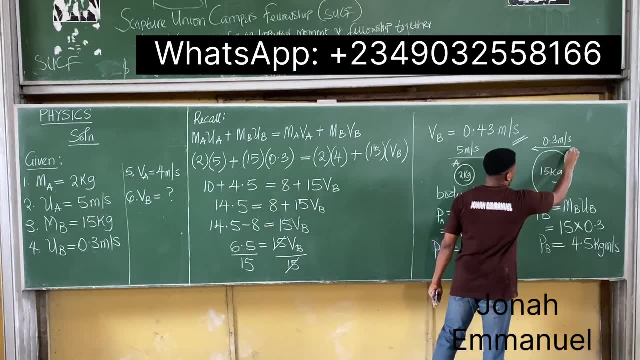 This is this, So we have this Alright. So if this is the case here, we can say that body A, this one here, this is body A, this is body B. We can say that body A has a greater momentum than body B. 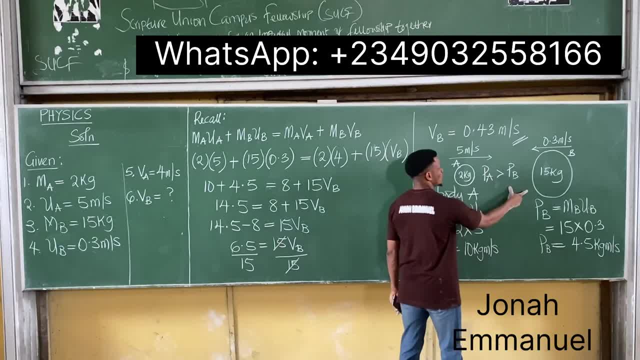 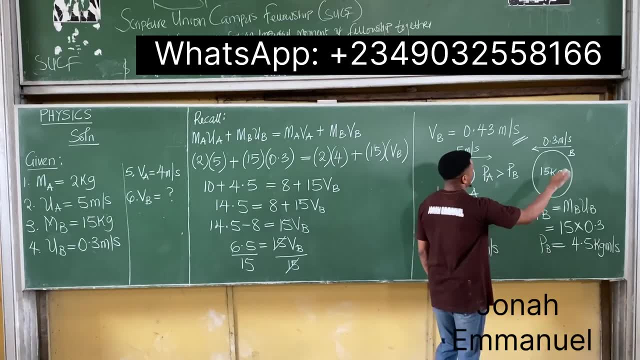 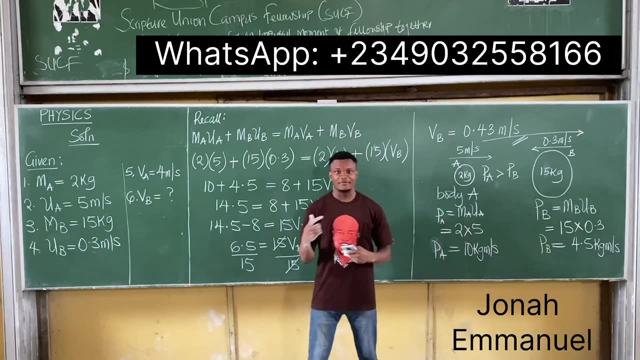 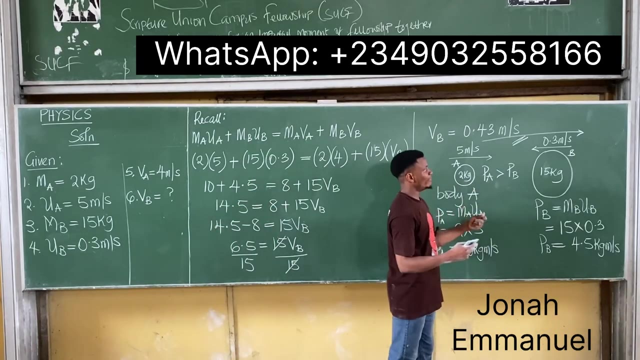 So if they collide, most likely they will both go in the direction of body A, Because body A has the greater momentum. So after collision the direction will go this way, the same as body A, And again this reiterates the idea that I shared earlier, when I said the direction that bodies will go after collision is not dependent on the mass of the body or of the size. 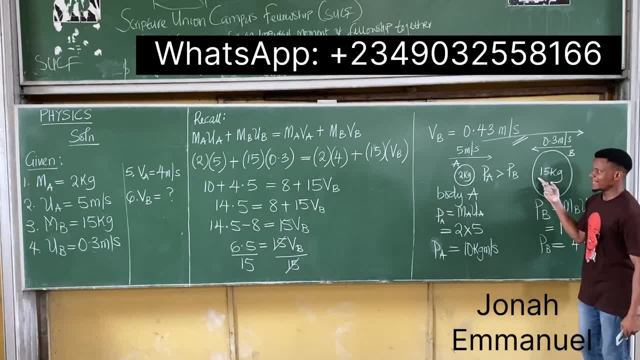 So you would think that since this man is 15 and this one is 2,, 15 is over 7 times of this. So this second body here, body B, has Over 7 times the mass of A. but then A is coming with a bigger momentum. 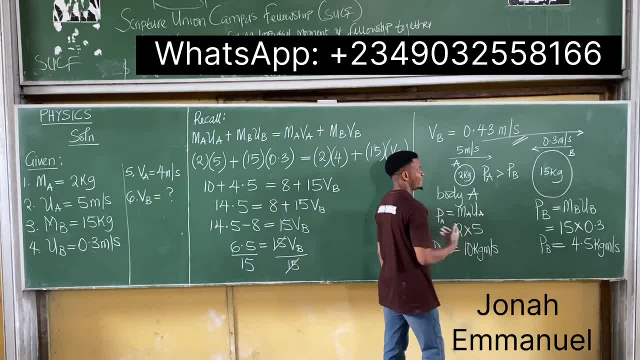 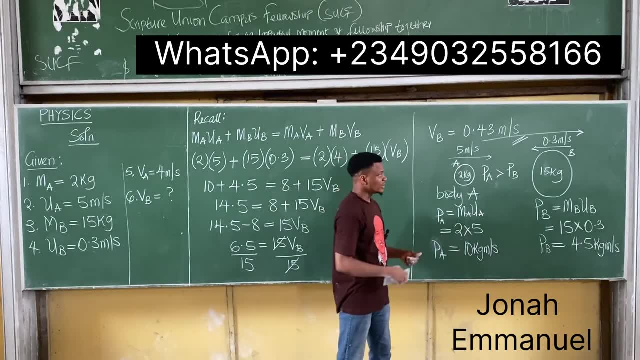 Why? Because it is moving with what there? A higher velocity, That's 5 as compared to 0.3. Alright, So most likely after collision the body might, The body would go in the direction of body A. So this is what you have here. 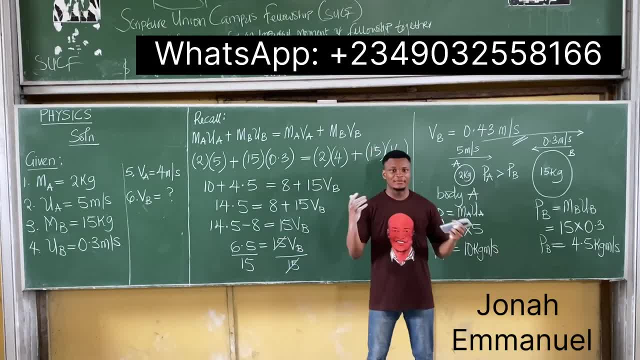 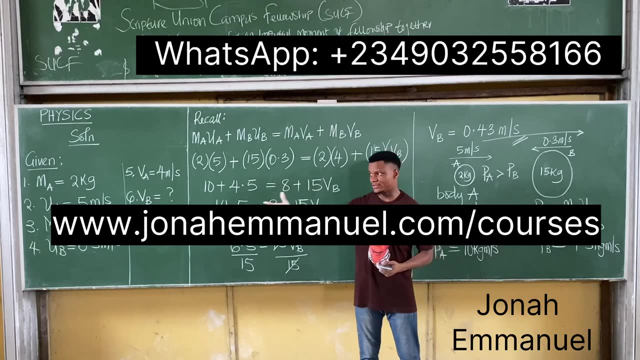 Alright, I prepared Um Over 50 videos on physics, chemistry and mathematics, So access my video courses for JAM and YX dance. Simply visit my website, wwwjohnaimanocom. forward slash courses And you see the course for YX, JAM, slash, YX classes.